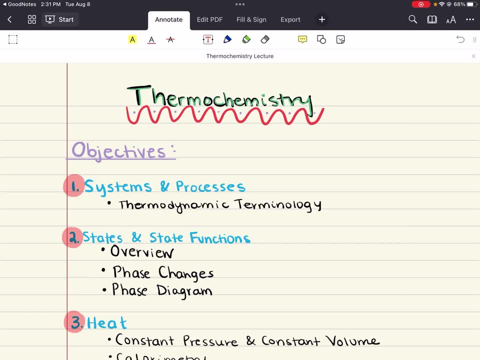 Hello everybody, my name is Iman. Welcome back to my YouTube channel. Today we're going to be discussing thermodynamics for MCAT, General Chemistry. Here we're going to cover the following objectives: First, we're going to talk about systems and processes. Here we're going to 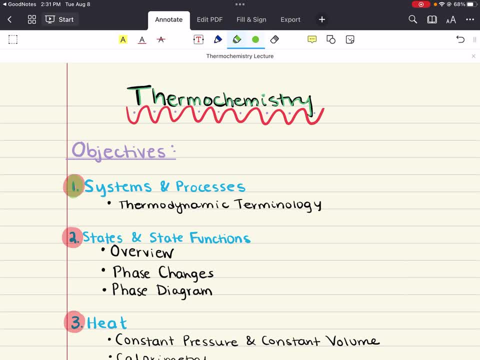 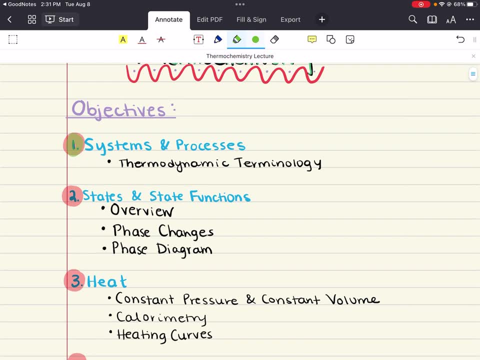 identify, or learn to identify, the system and the surroundings, given a situation that involves transfer of heat, And we're also going to define the features of a isothermal, adiabatic, isobaric and isochoric process. Then, in the second objective, we're going to talk about 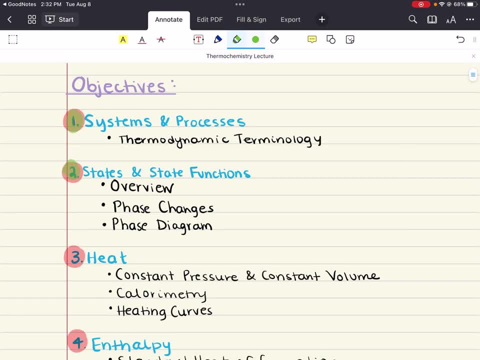 states and state functions. We're going to talk about standard conditions and the calculations they're used for. We're also going to distinguish between a state function and a path or process function, And we're going to list the common state functions as well, since those are important. 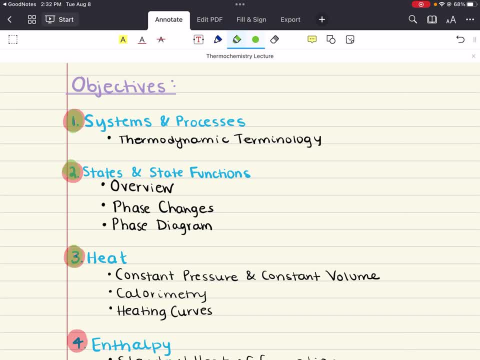 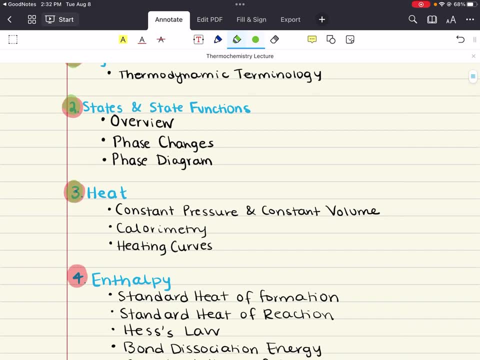 to remember for the MCAT. Our third objective is all about heat. We're going to differentiate between temperature and heat, We're going to compare specific heat and heat capacity, And then we're also going to make mention of the specific heat of water. 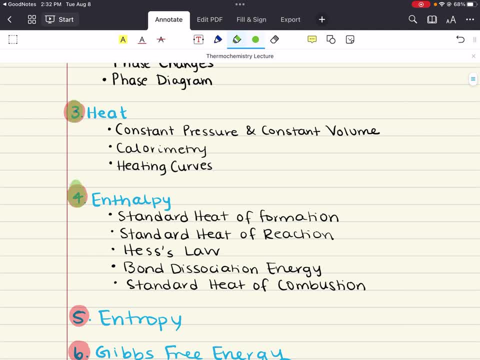 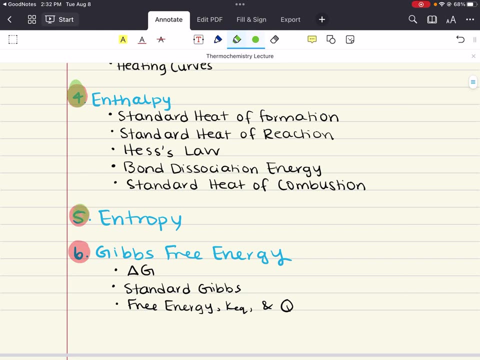 All right, then. the fourth objective is enthalpy. Here we're going to distinguish between endothermic and exothermic reactions, as well as define what enthalpy is and the enthalpy of a molecule or atom, given some reaction data. Fifth, we're going to move into entropy. Here we're going to define 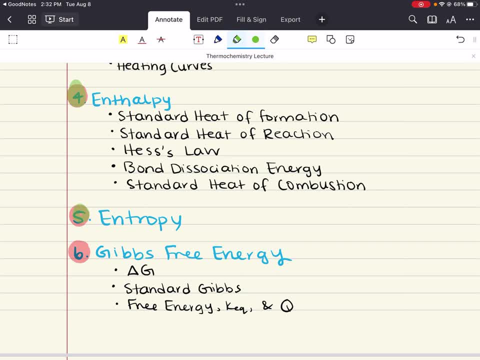 entropy and we're going to define it in terms of its relation to energy distribution and disorder. We're also going to order the phases of matter from lowest to highest entropy and learn to predict the direction of change in entropy within a given direction or within a given reaction. And then 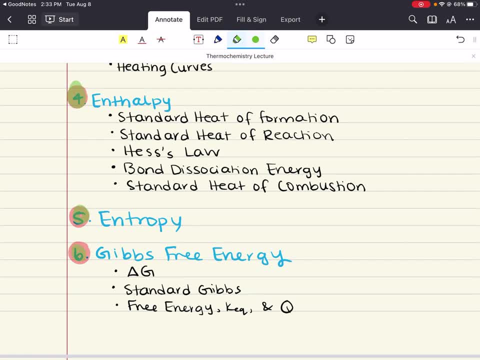 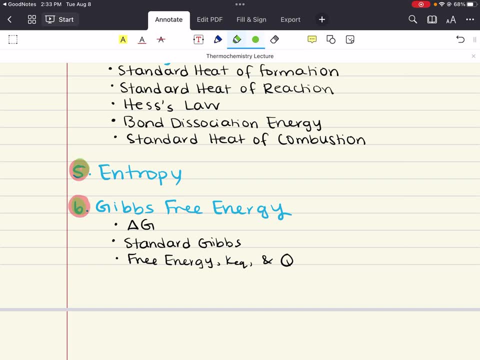 next and the final objective is going to be Gibbs free energy. So we're going to define Gibbs free energy. we're going to learn the equation for Gibbs free energy and then learn to determine the Gibbs free energy for a reaction at varying temperatures. We're also going to learn how to 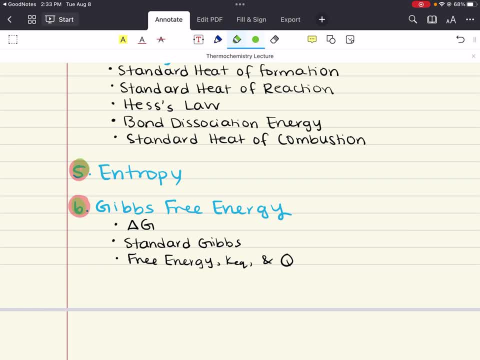 quantify how changing concentrations of reactants or product will alter the progress of a reaction and also temperature, And so that kind of encompasses all the main things that we're going to discuss in this chapter. Alright, it's a lot, but we're going to take it slowly, one piece. 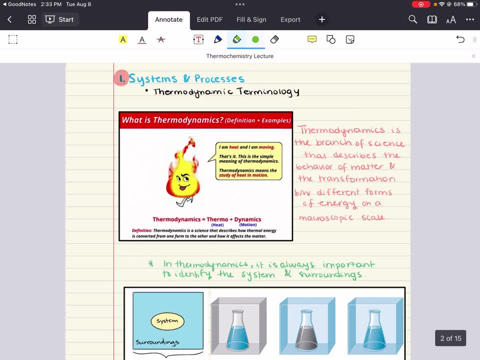 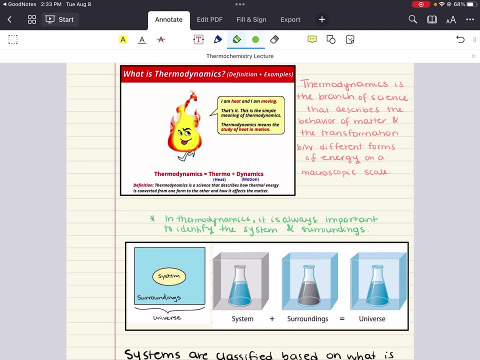 at a time. So let's go ahead and get started with that first objective. All right, let's define systems versus surroundings Now. a system, in scientific context, is a specific portion of the universe that is being observed or examined. All right, the system could. 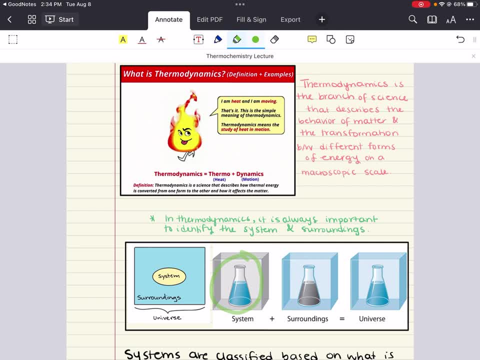 be any collection of physical or chemical entities, for example, all the reactants and products in a chemical reaction, or the solute and solvent in a solution, or even just the gas inside a balloon. Alright, so that system is a specific portion of the universe that you are observing or examining. 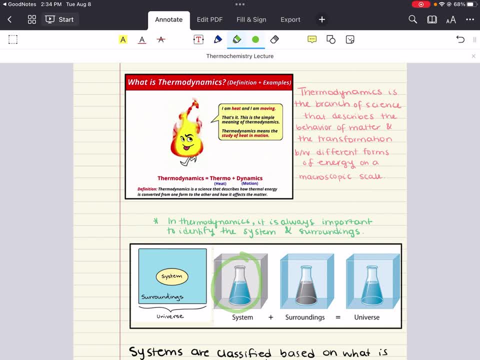 So let's say: we're only interested in the beaker, So the beaker is your system. Everything in the beaker, including the beaker, is our system. We can define it this way Now. conversely, the surroundings, also known as the environment, include everything. 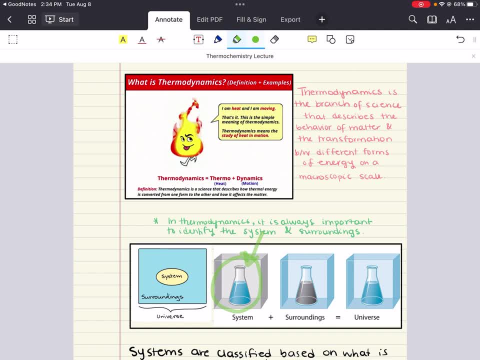 else outside of the system. Essentially, it's the rest of the universe that is not part of the system. So the system is the beaker. Everything else outside of the beaker is the surroundings, And together they make up the universe. Now you can. 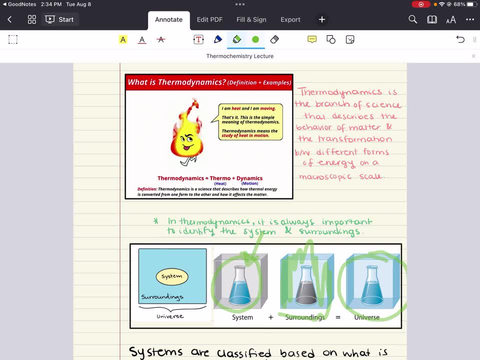 be even more specific. right, Your surroundings can be even more specific. So it could just be the room that you're in, that you're working under, for example. all right, So you can define the surroundings to be a lot more specific as well, All right. but generally we say: 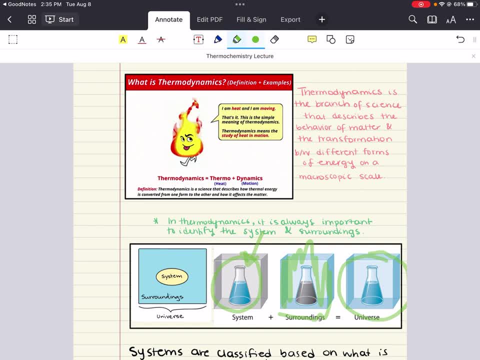 system is the specific portion of the universe that's being observed or examined, and the surroundings is known as the environment. It includes everything outside of the system. You could also limit that. Now the boundary- the boundary between the system And the surroundings- can be defined according to the observer's or experimenter's needs. 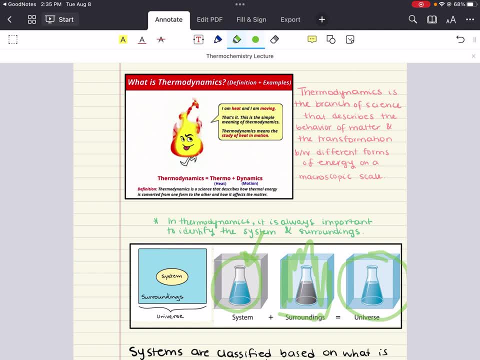 So, for instance, if you were studying, all right, the heat transfer from a cup of hot coffee, all right, to its cup, The coffee would be defined as the system and the cup could be defined as part of the surroundings. Now, if your focus is just on the heat exchange between the coffee cup system and the air around it, 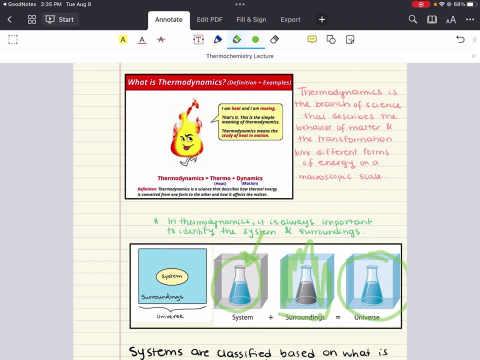 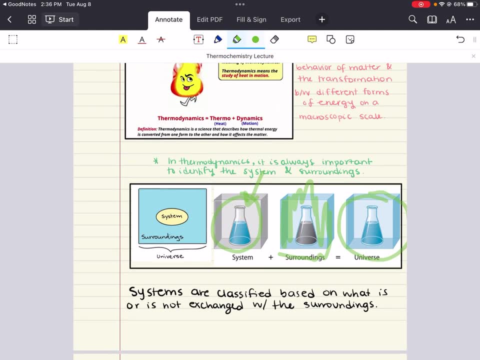 then both the coffee and the cup would be considered the system, And then the surroundings would be the air, all right. So, again, like we said, you can define your system and surrounding based off of your needs, what you're trying to observe, what you're trying to experiment on, all right. 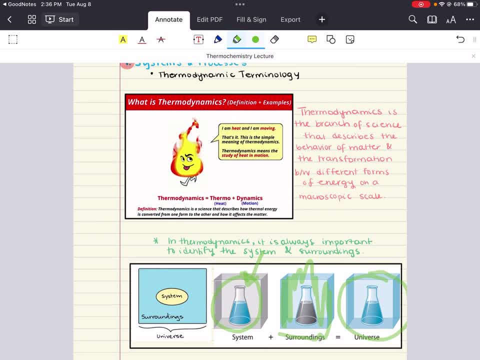 And so I think this is a good introduction to then introduce you to the definition of thermodynamics. It's this branch of science that describes the behavior of matter and the transformation between different forms of energy on the macroscopic scale. all right, Thermal heat dynamics- motion. 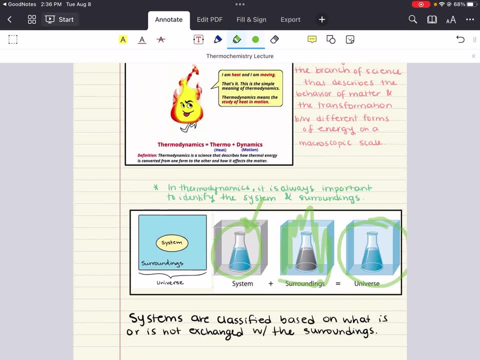 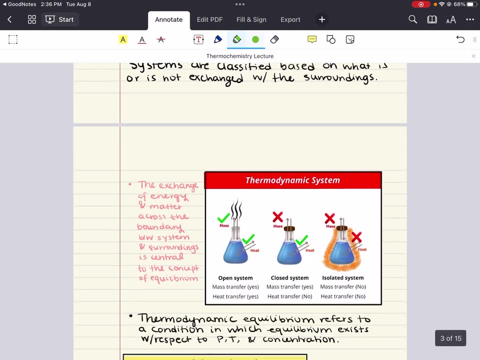 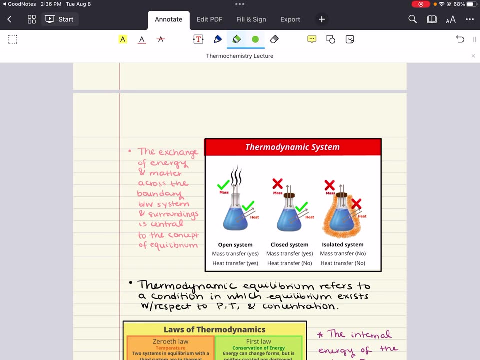 So you can think of it as heat motion. all right, Now, based on the interaction with the surroundings, your systems are typically classified, actually, into three categories. all right, You have three categories. You have isolated systems, closed systems and open systems. 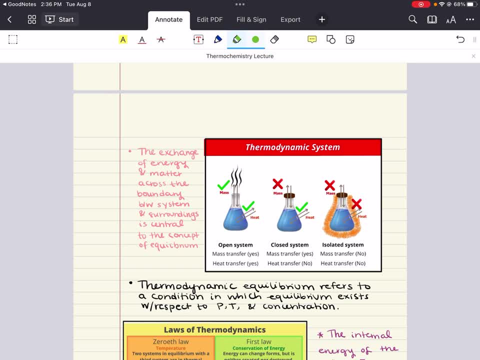 Isolated systems. These systems can cannot exchange energy- all right, In the form of heat or work, And they cannot exchange matter with their surroundings. all right. So isolated systems cannot exchange energy or matter with their surroundings. Then we have closed systems, all right. 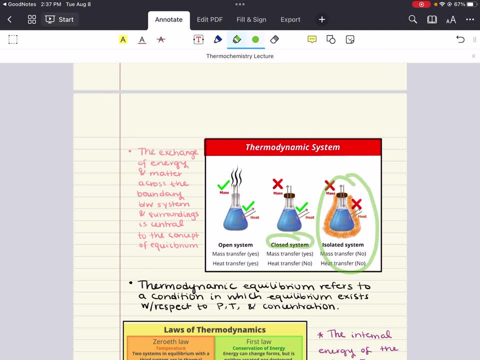 These systems can exchange energy, all right, But not matter with the surroundings. all right, They can exchange energy, but not matter with the surroundings, And I always think that this figure has it a little bit twisted up. all right, Closed systems can exchange energy, all right. 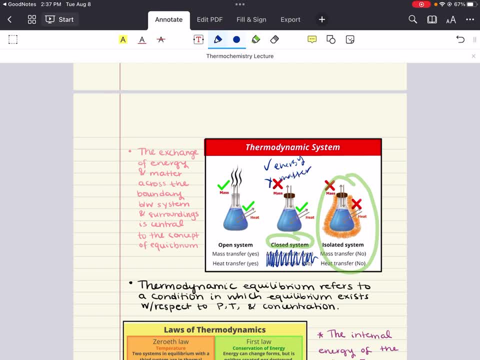 But they cannot exchange matter. all right, Fantastic. What about open systems? As the name implies, these systems are open. They can exchange both energy and matter with the surroundings. all right. So those are our three types of systems Based on the interaction between surroundings and systems. 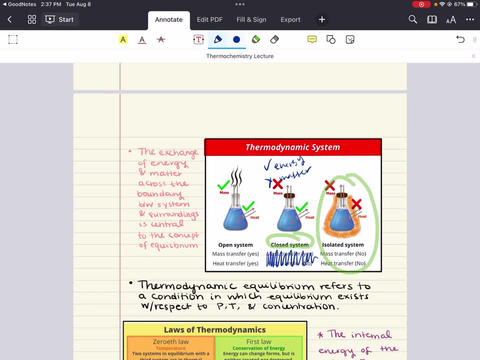 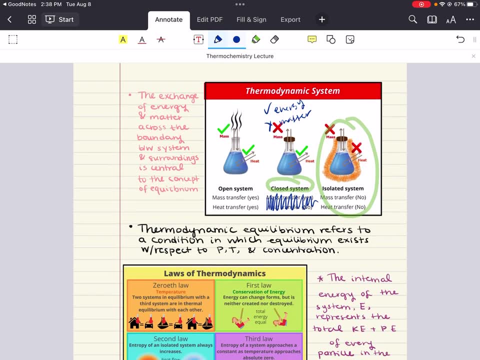 we have these three categories: all right, Open, Closed And isolated. Now a process in general is defined right As a change in the state of a system. all right, A change in the state of a system. It's marked by a change in one or more of its properties. 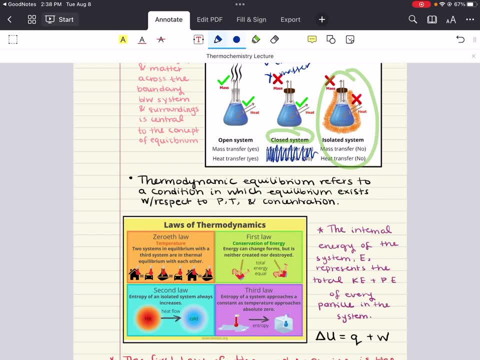 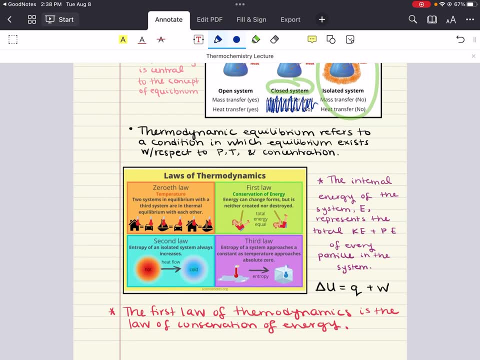 These properties could include concentration of reactants or products. It can include temperature or even pressure. Certain processes are uniquely identified by some property that remains constant throughout the process. These conditions often allow for the simplification of the first law of thermodynamics, The first law of thermodynamics. it can be expressed mathematically, all right. 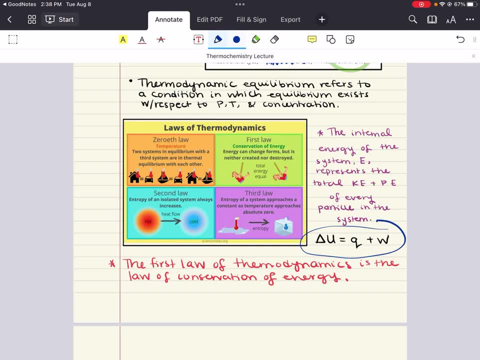 With this equation, Delta U represents the change in internal energy of the system. all right, That is equal to the heat plus work. It is equal to the heat added to the system and the work that is done by the system. Each of these elements, they play a crucial role. 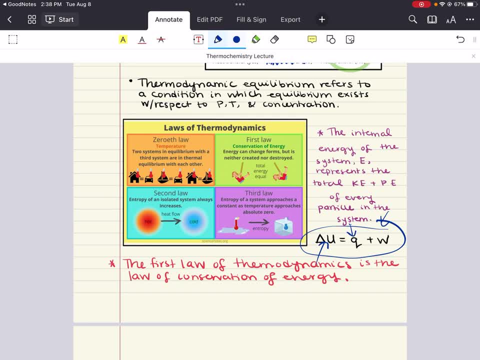 Each of these elements, they play a crucial role. Each of these elements, they play a crucial role in defining the behavior of systems in thermodynamics. all right, So that's a mathematical definition of the first law of thermodynamics, But let's go into a little more detail, all right. 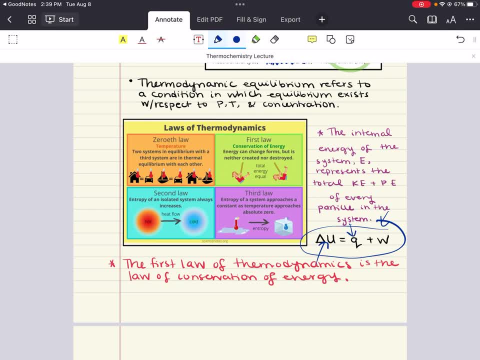 Conceptually, what is the first law of thermodynamics? Well, the first law of thermodynamics is also known as the law of energy conservation, all right. And it states that energy cannot be created or destroyed in an isolated system. all right. The total amount of energy that is created in an isolated system is the total amount of energy that is created in an isolated system. The total amount of energy that is created in an isolated system is the total amount of energy that is created in an isolated system. 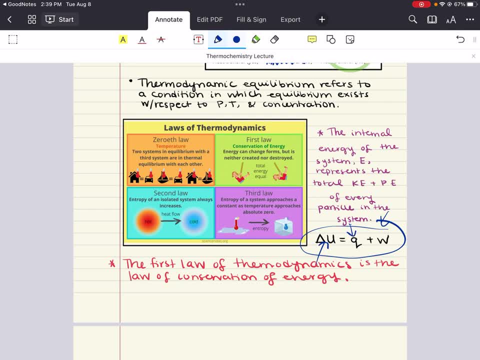 The total amount of energy and matter in the universe. it must remain constant, all right, But it can change from one form to another. So you cannot create energy or matter, but you can transform it, all right. So, in essence, energy can be transferred or transformed from place to place, or transformed into different forms. 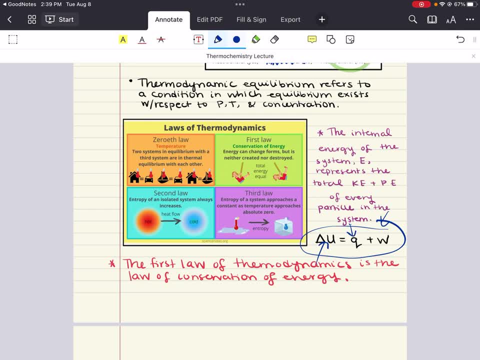 It just cannot be created or destroyed. all right, Now this equation. it tells us something. It essentially says that any increase in the internal energy of a system, delta U, is due to the transfer of energy, due to the heat that may be added to the system q and or the work done on the system by the 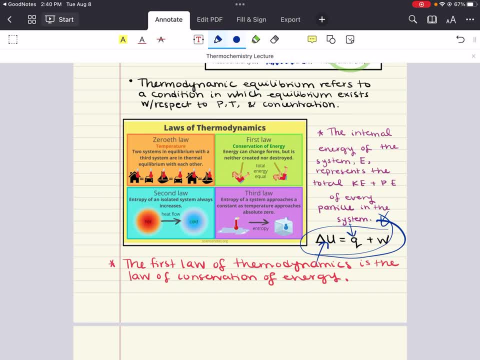 surroundings. that's the w. all right, so it tells us: all right, change in internal energy, an increase. all right, what? what can result in that increase? some heat change, some work change. all right, now, that's the first law of thermodynamics. now we can also recall which is going to be very 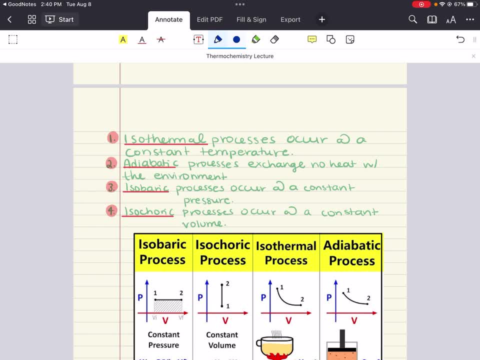 important for us to understand. um we can recall the features of isothermal, adiabatic, isobaric and isochoric or isovolumetric. those are synonymous processes. all right, so isothermal, we need it. all right, isothermal, adiabatic, isobaric or isochoric, and this is also known as isovolumetric processes. 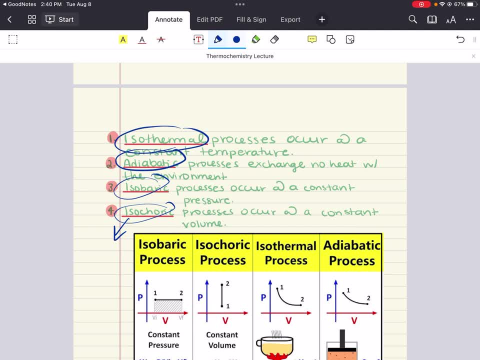 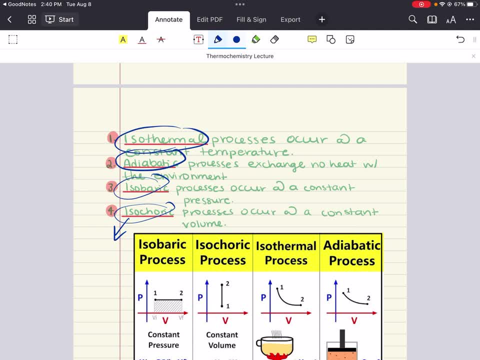 on a conceptual problem in relation to these four features, these four processes all right. what is an isothermal process, first and foremost? well, an isothermal process all right is where the temperature of the system remains constant. this means that the system's internal energy also remains constant. right, because internal energy is directly proportional to temperature. 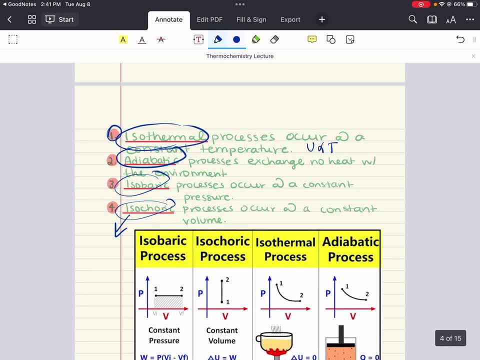 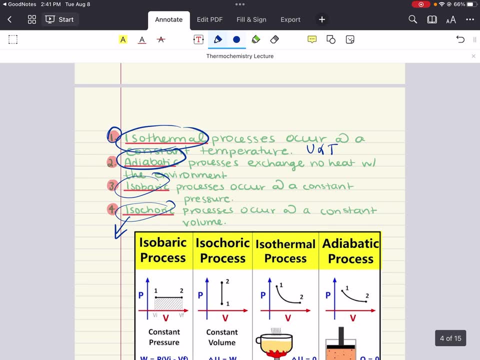 that's an important relationship, directly proportional to temperature. you can't see it in this equation, all right. but if you take physical chemistry, all right, you will work through why. internal energy is related to temperature, all right, the mathematics at least, all right. but internal energy is directly proportional to temperature. so in an isothermal, 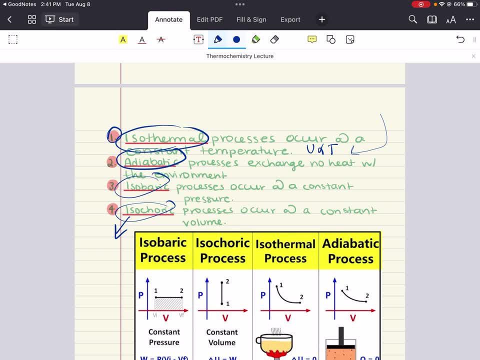 process, the temperature of the system remains constant, and that means that the internal energy also remains constant. now, a good example of this is: the temperature of the system remains constant. now, a good example of an isothermal process is your ideal gas expansion or compression. where the system is in contact with some heat reservoir, that ensures constant temperature. all right, and then? 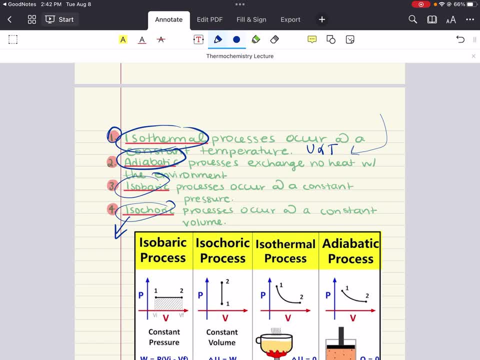 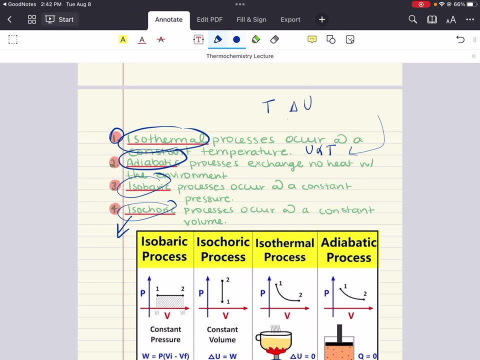 from the first law of thermodynamics for an isothermal process, all heat added to the system is converted into work done by the system. all right, because temperature stays constant, delta u stays constant, or or u stays constant, so delta u is equal to zero. if delta u is equal to zero, then q plus w is also equal to zero, so then you can write a relationship. 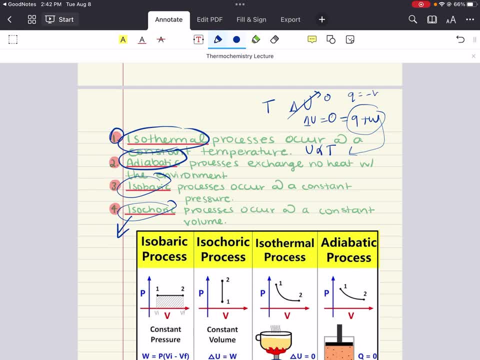 between heat and work, q is equal to minus work. all right, so from this first law of thermodynamics for an isothermal process, all heat that's added to the system is converted into work done by the system. fantastic, then second, we have our adiabatic process. 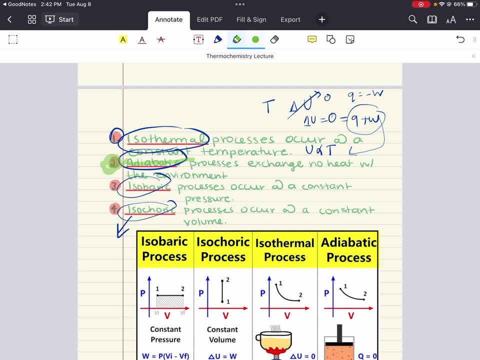 an adiabatic process is one where no heat is exchanged between the system and its surroundings. so in other words, the system is thermally insulated from its surroundings. so any work that's done on or by the system is just going to result in a change in the internal energy. 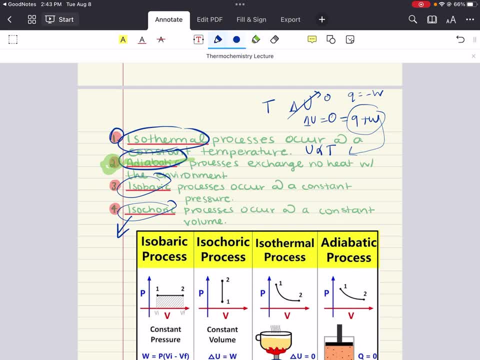 of the system. so for an adiabatic process, all right for an adiabatic process, since no heat is being added or removed, q is equal to zero. all right, q is equal to zero, and so delta u is just equal to work. all right, fantastic, then we have isobaric. 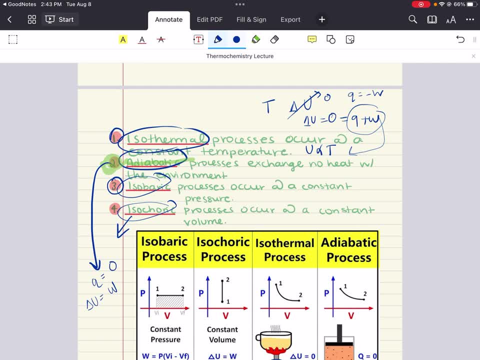 process. in an isobaric process the pressure of the system remains constant. so under this condition any heat added to the system is going to be partially used to do work, by expanding the system if the volume increases and partially increasing the internal energy if temperature increases. now, unlike other processes, here both heat and work interactions can occur in an 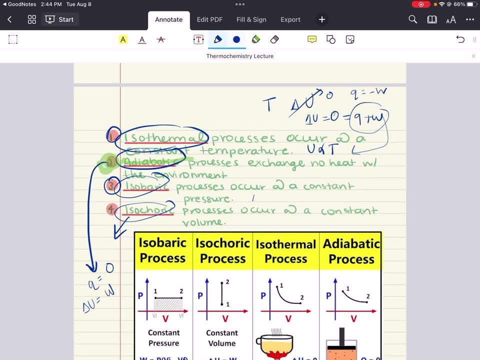 isobaric process. so nothing really changes in your equation for your internal energy. all right, fantastic. then we have, last but not least, an isochoric process. in an isochoric process, which is also known as an isovolumetric process, the volume of the system remains constant. 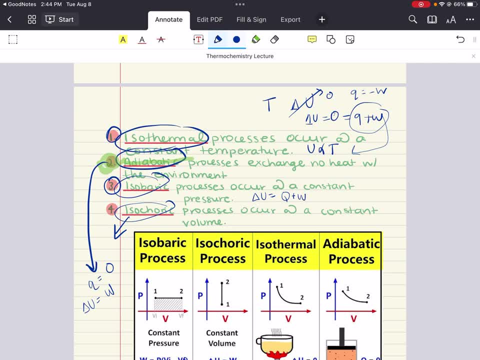 this means that no work is done by or on the system, since work often involves a change in volume. remember, we've defined work to be equal to pressure times, delta v. but if nothing is changing with the volume, then delta v is just zero, all right, which means work is zero, and so then internal. 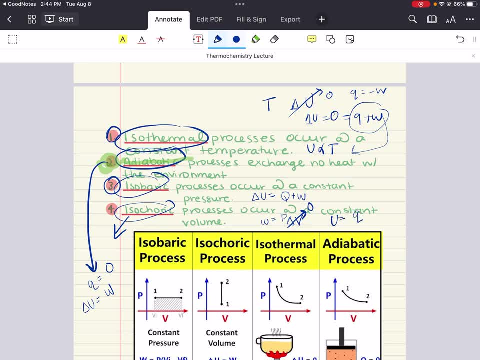 energy is equal to q for an isochoric process. fantastic, remember, in actual physical situations many processes are done by the system in an isobaric process, so no heat added to the system. they do not fall neatly into one of these categories, but they're more of an approximate. 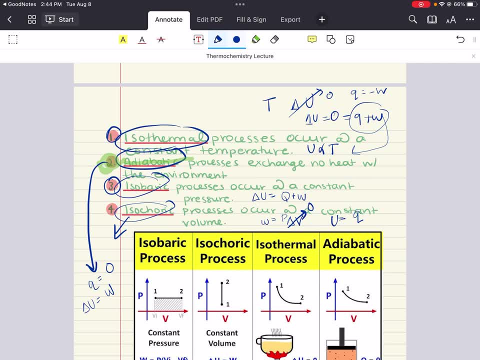 of them. under certain conditions, all right. but these idealized processes- isothermal adiabatic, isochoric, isobaric- are extremely useful in developing the theory and understanding of thermodynamics, which is why we talk about them and why we define them. now we have our graph here that 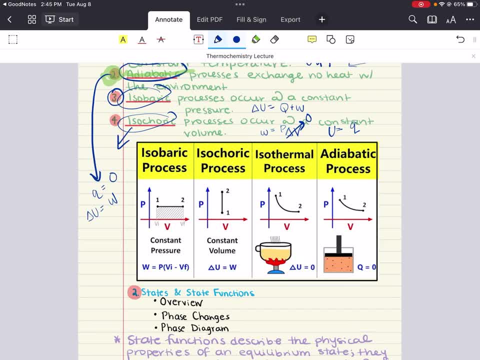 summarizes this and what it would look like in graph form in a pressure versus volume graph. so in an isobaric process: all right, pressure doesn't change. all right, so you usually see this as a straight horizontal line on a pressure versus volume graph. all right, then, in an isochoric process. 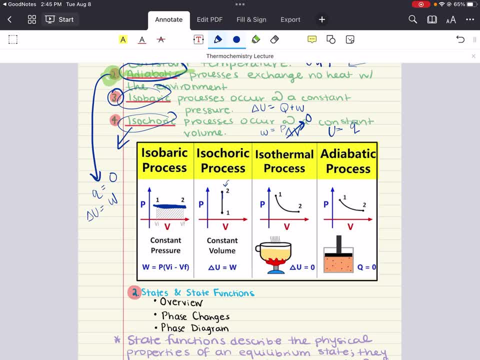 volume doesn't change, all right, but pressure does. so you have a vertical line in an isothermal process, all right, temperature stays the same and so does delta u, and so you see this kind of as a curve, because now, uh, because now pressure doesn't change all right. so in an isobaric process you 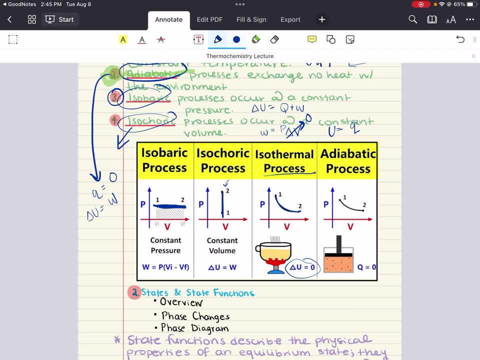 and heat equal to each other. all right, And in a pressure versus volume graph you're going to see it as a curve of some sort. In adiabatic processes, Q is equal to zero because there's no heat transfer. all right, And so in your pressure versus volume graph you'll also see some sort 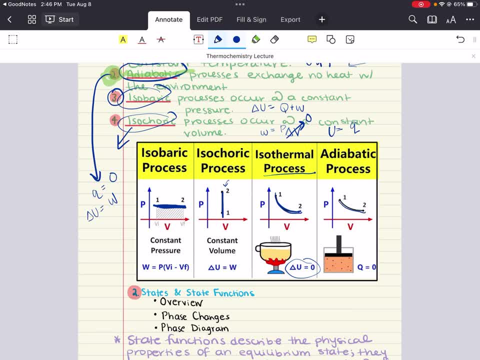 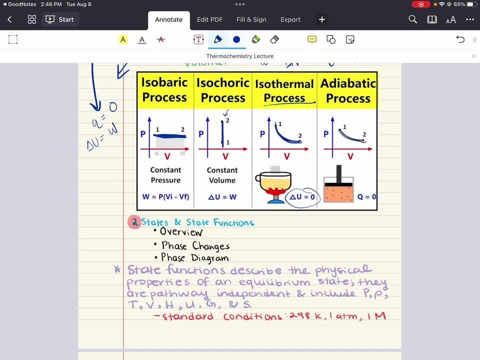 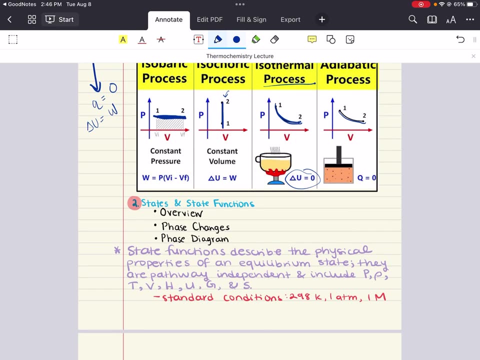 of line or curve as a representation of this adiabatic process. all right With that. all right With that, we can move into our second objective. all right, We can move into our second objective. I do want to define one thing very quickly that we're going to elaborate on in the 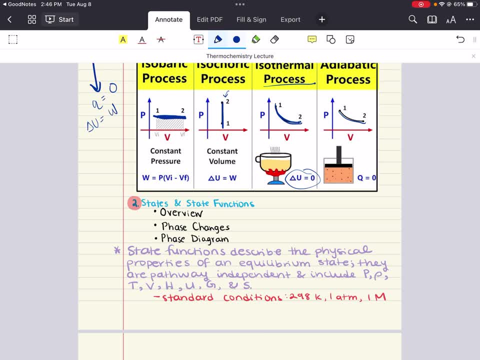 last objective when we talk about Gibbs: free energy. but I think it's important to state earlier: all right, In thermodynamics, a process can be either spontaneous or non-spontaneous. all right, A spontaneous, Spontaneous process is the one that can occur without the need for external energy input. 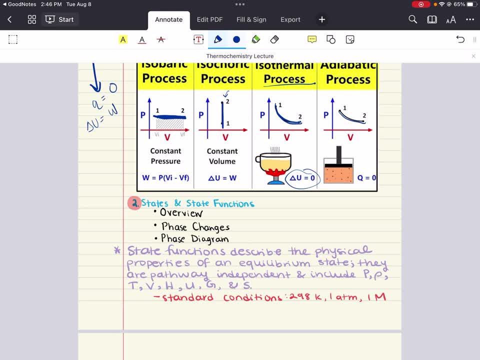 whereas a non-spontaneous process requires an outside energy source for it to take place. all right, Now, the thing that's important to understand, and why I want to make mention of this, is because in the previous chapters we talked about kinetics: how fast a reaction proceeds. 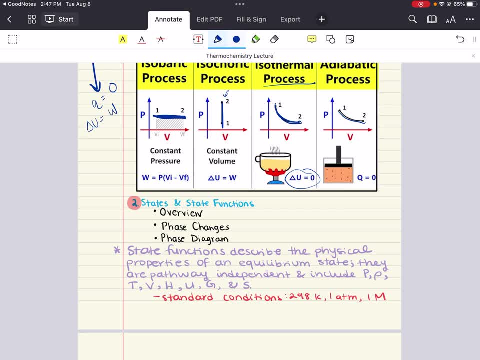 When we're talking about thermodynamics, we talk about spontaneous or non-spontaneous, whether a reaction can happen without input energy or not, all right. And it's important to understand that spontaneous doesn't necessarily mean instantaneous or fast, all right. That's not a relationship you should. 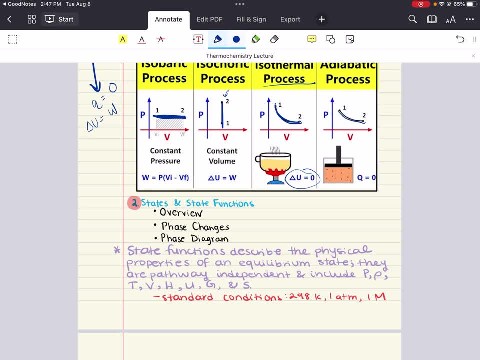 make A spontaneous reaction actually might not happen quickly, all right, And it may not go to completion, but the definition means that it does not require an outside energy source for it to take place, all right. So in the case that we make mention of Gibbs, free energy or the term 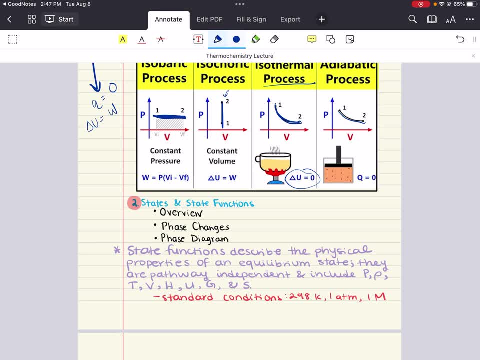 spontaneous and non-spontaneous. we're going to talk about kinetics and we're going to talk about spontaneous. It's just important to distinguish between thermodynamics and kinetics, first and foremost, and also not to associate the word spontaneous with instantaneous or quickly. 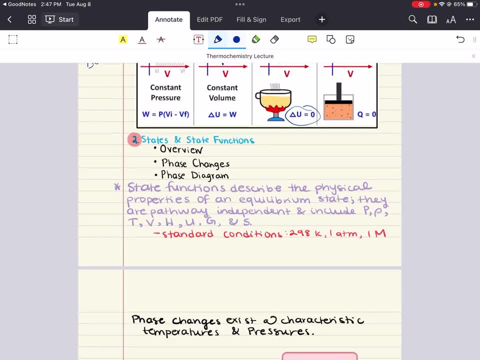 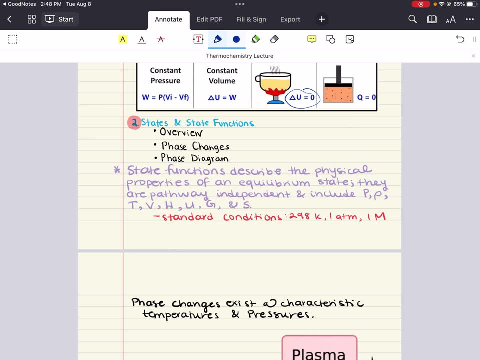 all right, With that little spiel. now we can officially move into the second objective. all right, Here we're going to talk about states and state functions. Now, in thermodynamics there are two kinds of properties used to describe systems: state functions and path functions. 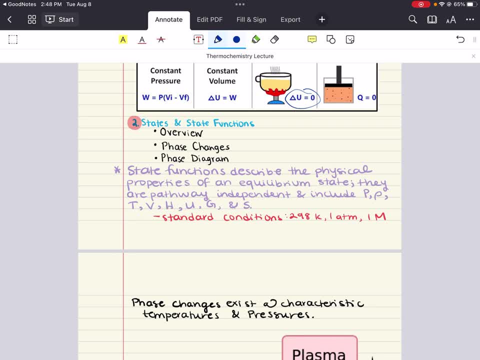 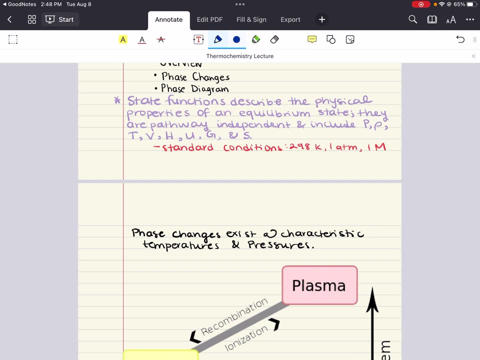 also sometimes called processes. The key difference between the two lies in their dependence, or lack thereof, on the path that's taken to achieve a state all right State functions. State functions are properties that describe the state of a system in equilibrium, and they really only depend on the current state of the system. 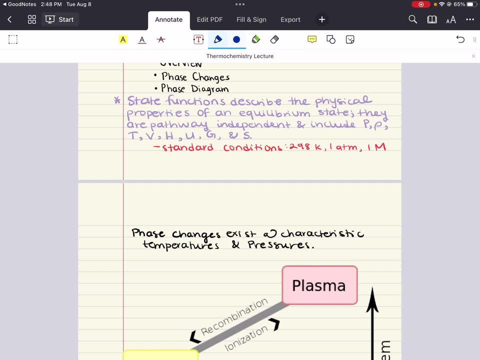 and not how the system arrived at that state. So they're really useful for comparing different equilibrium states because they're not just the state of the system, they're the state of the system. Their values only depend on the initial and final states of a system, not the path taken. 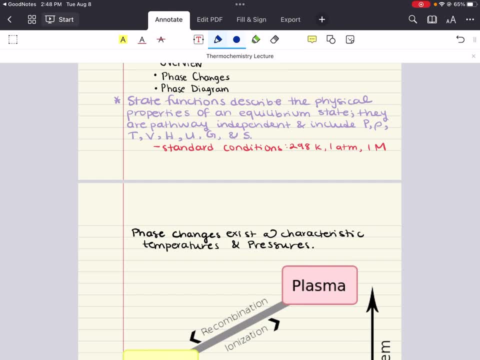 to get from one state to another. all right. That is what a state function is. Examples of state functions include: all right. pressure, density, temperature, volume, enthalpy- all right. internal energy, Gibbs, free energy and entropy- all right. 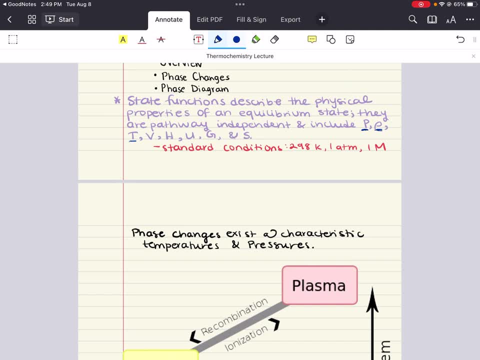 So that's what all these letters are: pressure, density, temperature, volume, enthalpy, internal energy, Gibbs, free energy and entropy- And actually a really fun one. you know I usually don't like mnemonics personally. that's just a personal choice. 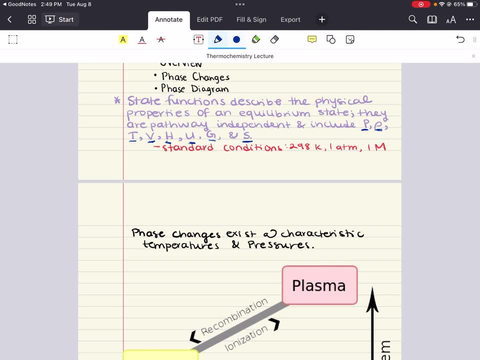 I think when you're studying for a test like the MCAT, maybe there's just too many mnemonics and a lot of students end up confusing their mnemonics, or because there's so many to memorize, it becomes hard, And so you know there's a lot of things that you can do to. 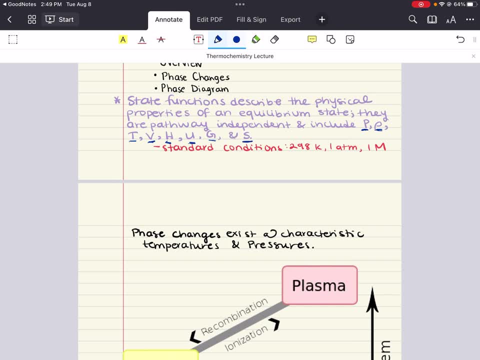 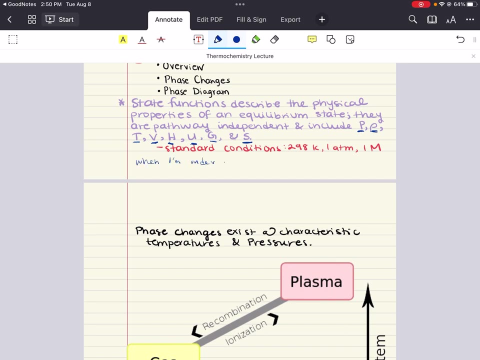 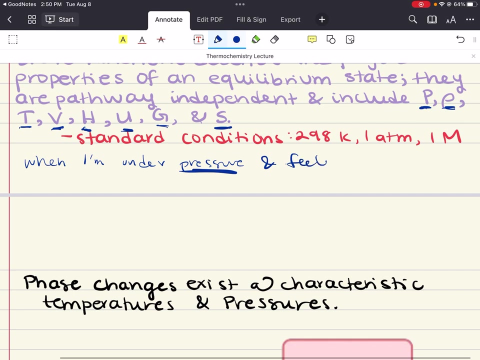 I will say that my favorite mnemonic is the one that helps you remember state functions- all right, And the mnemonic is when I'm under pressure and feeling dense- all right. When I'm under pressure and feeling dense, all right. All I want to do is 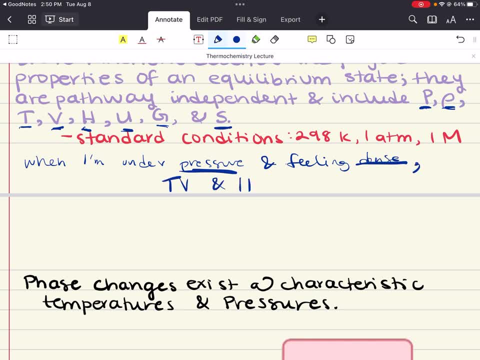 is watch TV and get hugs, all right. So this helps you remember all your state functions. pressure- ooh, where's my highlighter. Pressure, density, temperature, volume, enthalpy, internal energy, Gibbs, free energy and entropy. all right, This is the only mnemonic. 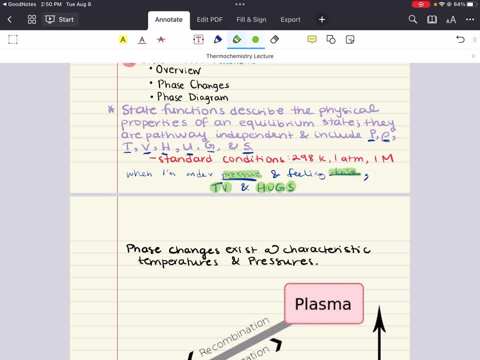 that I support. personally, I think all the other ones are a little bit too much, all right. And memorizing too many mnemonics: I think it's a little bit too much, all right. And memorizing too many mnemonics: I think it's a little bit too much, all right. And memorizing too many. 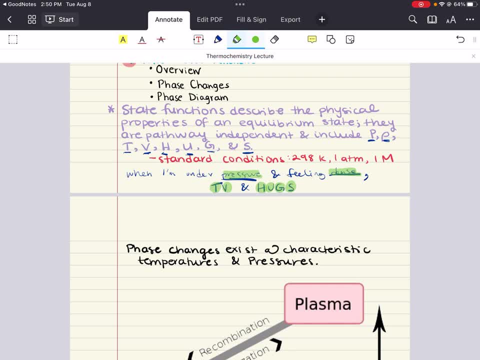 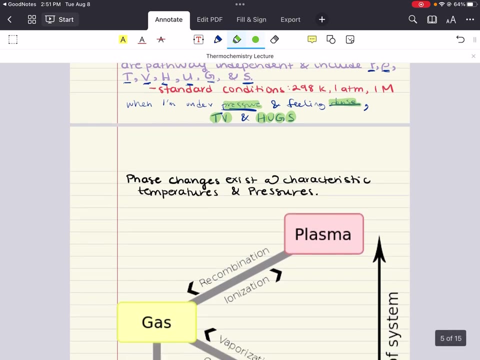 mnemonics can also very much get in the way of understanding and remembering the content itself. all right, But that is such a subjective thing to say. all right, That is just an opinion. all right, So that's state functions for us. before I get too much into my opinions on things, 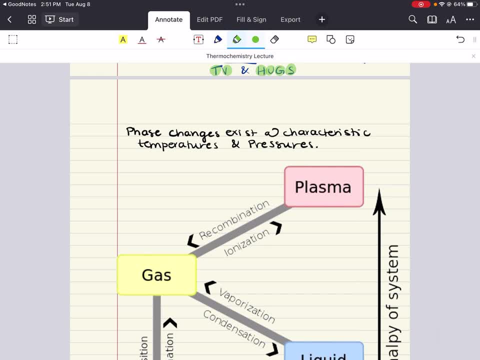 which don't matter here. all right. So then path functions. what are path functions? All right, we said state functions, all right. Properties that describe the state of a system and they only depend on the current state of the system. All right, so we said state functions, all right. 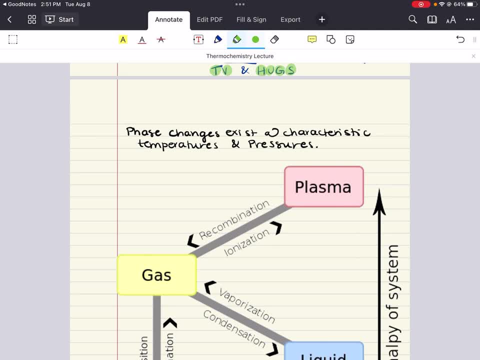 Not how the system arrived at that state. Path functions. on the other hand, these are properties that depend on the route taken to achieve a state, So they describe the process of the system. In other words, they provide information about how that system got to its current state And the most 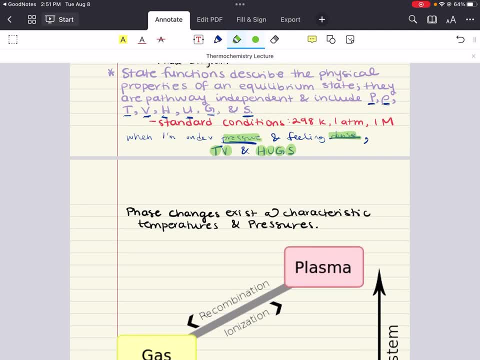 important path functions. all right, the most important path functions that you should know are work and heat. All right, these are two examples of path functions. The values of these functions- heat and work- depend on the specific transition or path that a system takes. 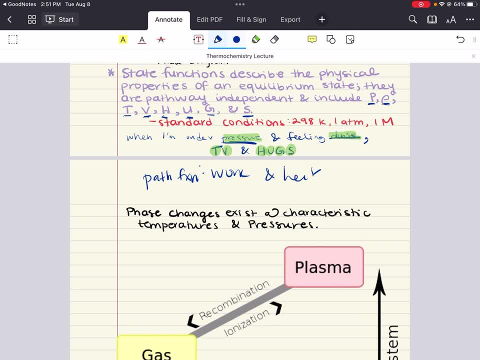 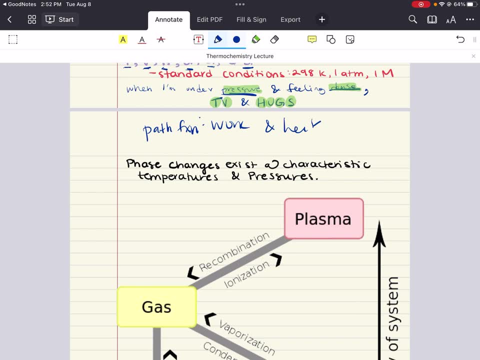 to get to its state, all right. to get from one state to another, All right. fantastic. So that is the difference between state and path functions. All right, make sure you remember what falls under which path. Now, because systems can be in different equilibrium states at different temperatures. 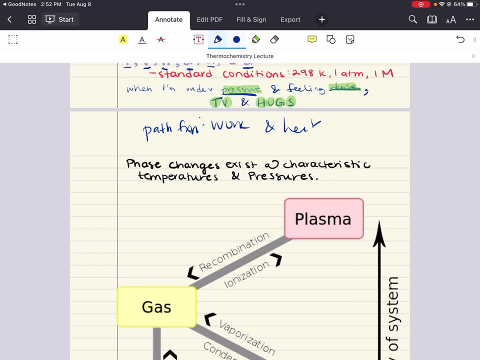 and pressures. a set of standard conditions has been defined for measuring things like enthalpy, entropy and Gibbs free energy changes of a reaction. What are those state conditions? They're defined as 25 degrees Celsius. all right, And let's write this down in red Standard. 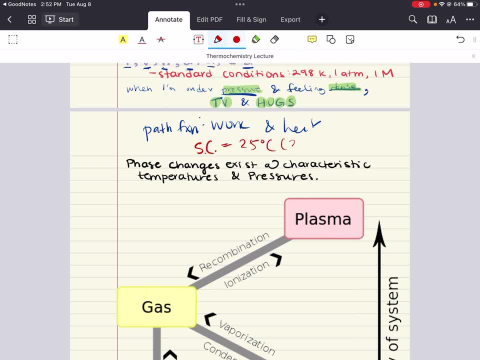 conditions is defined to be 25 degrees Celsius, all right, And let's write this down in red: 25 degrees Celsius or 298 Kelvin, all right. One ATM, one atmosphere pressure and one molarity, all right. Don't confuse standard conditions: 25 degrees Celsius, one ATM and one. 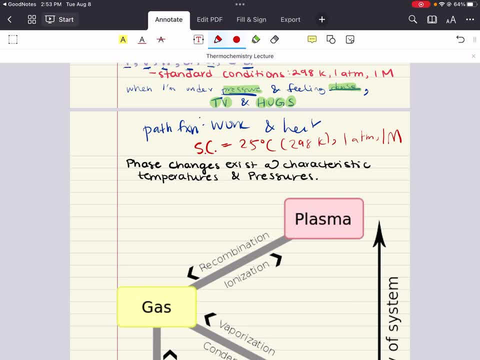 molar: all right. One molarity with standard temperature and pressure. STP: all right. That's something that we're going to define. when we talk about gases, which is, I think, the next chapter here, all right, And when we do that, we're going to talk about STP. This is not the same as the 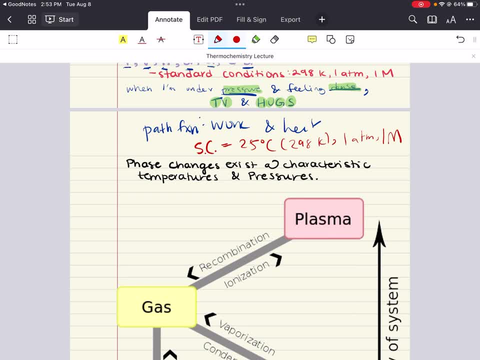 standard conditions, so do not confuse the two. Standard conditions are used for kinetics, equilibrium and thermodynamics problems. STP is only used for ideal gas calculations. Now, unlike standard conditions, the most stable form of a substance is called the standard state. 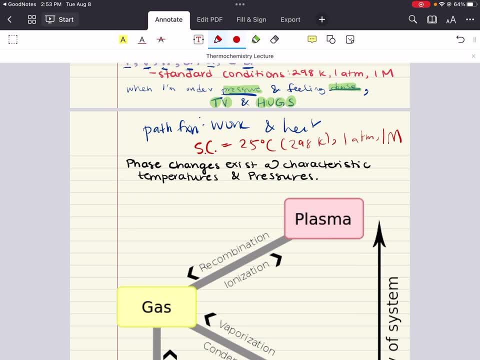 of the substance, all right, And the changes in enthalpy, entropy and free energy that occur when a reaction takes place under standard conditions are going to be called standard enthalpy, Standard entropy and standard free energy changes, and they're going to be symbolized. 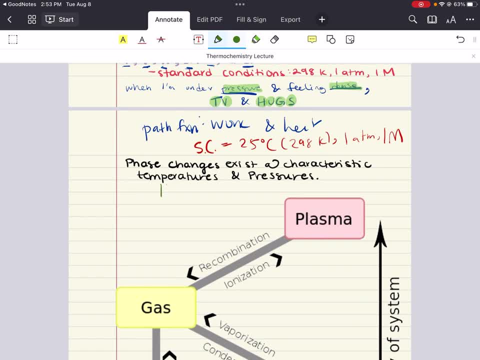 as the follow: So enthalpy is H, entropy is S, Gibbs free energy is G. When we talk about the changes in these conditions- enthalpy, entropy and free energy- that will occur when a reaction takes place under standard conditions. we call them standard enthalpy. 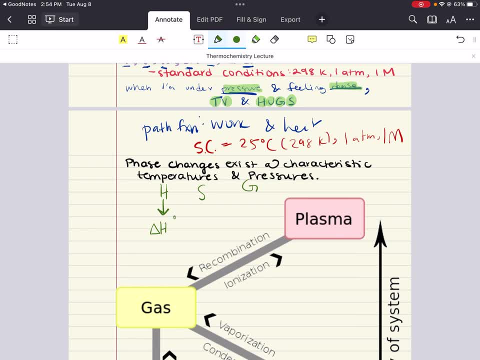 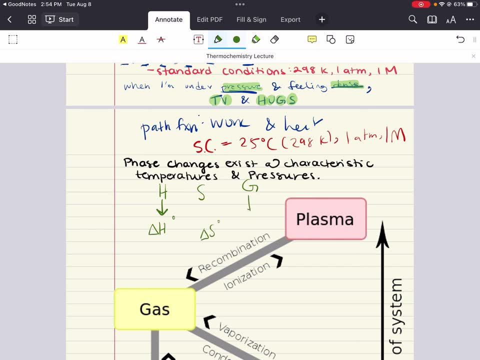 which is denoted as delta H, with a little degree sign. all right. For entropy, standard entropy, that's delta S with a little degree sign. all right, Delta S- naught, that's what I'm going to call it. all right. And for Gibbs: 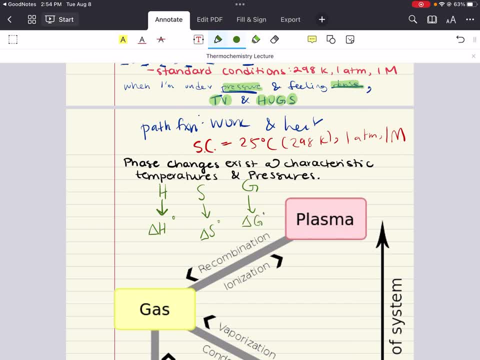 standard free energy, that's going to be delta G. little degree sign, all right. The degree sign in these variables represents zero, as the standard state is used as the zero point for all thermodynamic calculations. Now, keeping that in mind, we can start to talk about phase diagrams. 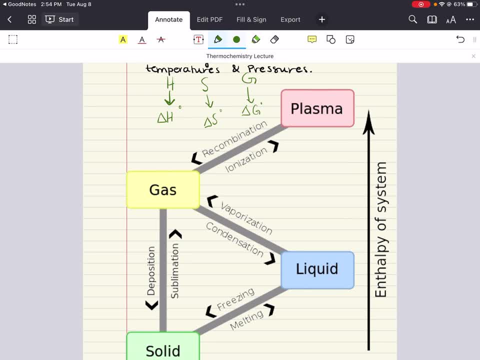 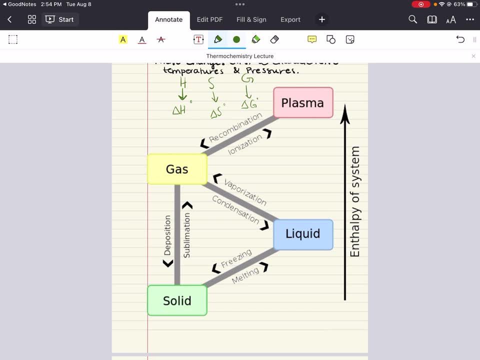 phase changes. all right, This is where things get interesting. Phase changes represent a transition between different states of matter, so solid, liquid and gas. Now we could also talk about plasma, but that's not of interest to the MCAT, so we're going to forego that conversation. 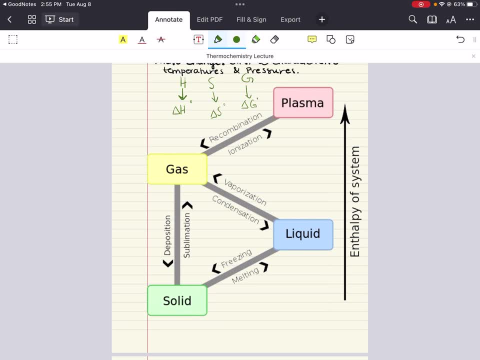 here, all right. But we can talk about changes between solid liquid and gas phase, all right. Now we can have a change between gas and liquid, all right. We can go from gas to liquid, for example. all right. If we go from gas to liquid, that's called condensation, all right. 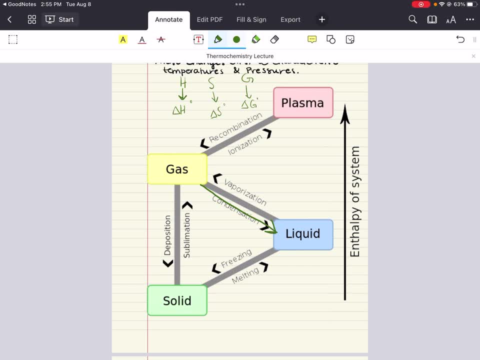 When a gas cools down, its molecules slow down, they start to stick together and they're going to form a liquid. This process is called condensation. The temperature at which this happens is called the boiling point. all right, BP, boiling point. Now you can also go the other. 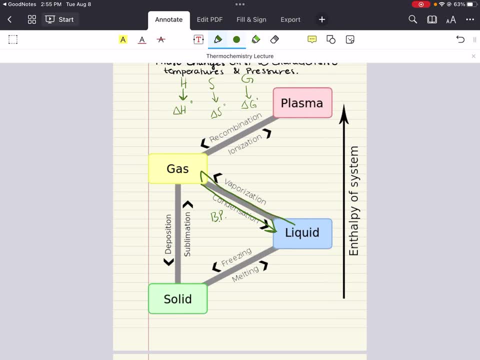 way You can go from liquid to gas. We call this vaporization. When a liquid heats up, its molecules move so quickly they break free of the liquid surface and they form a gas. This process is called vaporization or evaporation. If the vaporization happens throughout the volume of the liquid, then we call that. 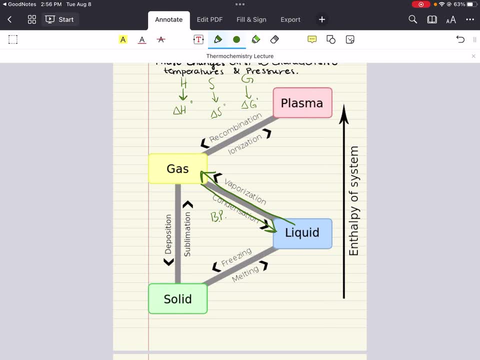 boiling. So the temperature at which this happens is called the boiling point. all right, So that's gas to liquid and liquid to gas. What about liquid, Liquid to solid? all right, What if we want to go from liquid to solid? We call this freezing. 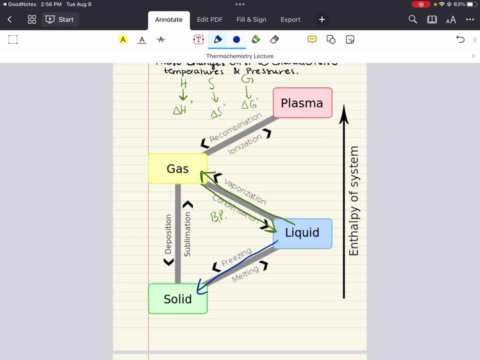 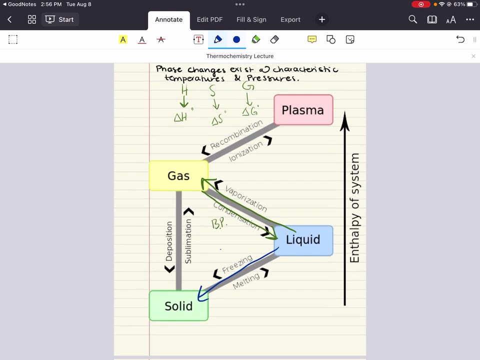 When a liquid cools down further, its molecules move so slowly that they begin to lock into place, forming a solid. This process is called freezing or solidification, and the temperature at which this happens is called. you guessed it, the freezing point. all right, What about if I want? 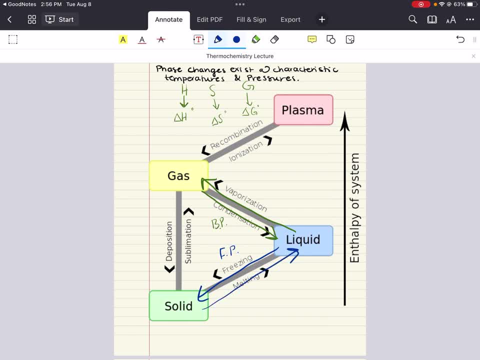 to go from solid back to liquid. If the vaporization happens throughout the volume of the liquid, this is called melting. all right, So you take your solid, you can heat it up, its molecules gain enough energy to break free from their fixed position and then they start. 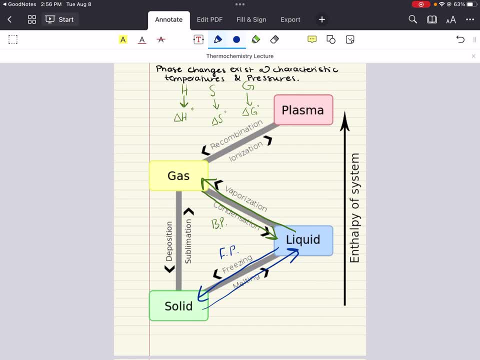 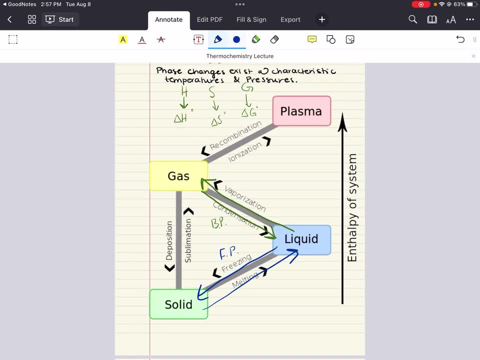 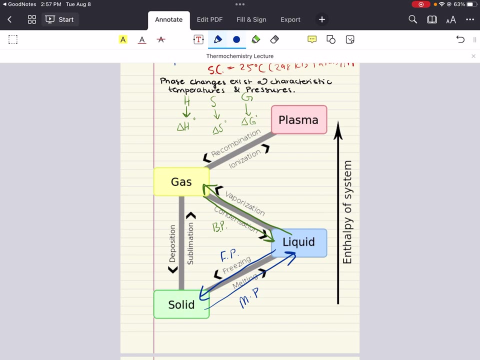 to move around, forming a liquid. This process is called melting or fusion, and the temperature at which this happens is called the melting point. all right, Melting, oh, melting point. all right, Cool, So that we've covered gas to liquid, liquid to gas, We've covered solid to liquid. 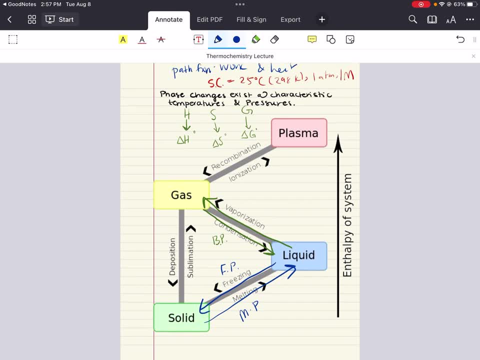 liquid to solid. We've covered. liquid to liquid. liquid to liquid. We've covered liquid to liquid. all right. What about solid to gas? All right. what if we want to go from solid to gas? We call this sublimation. In certain conditions, a solid can directly become a gas. 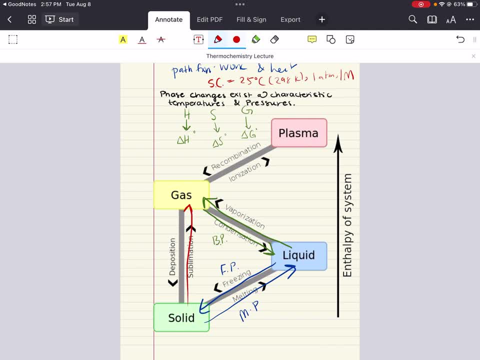 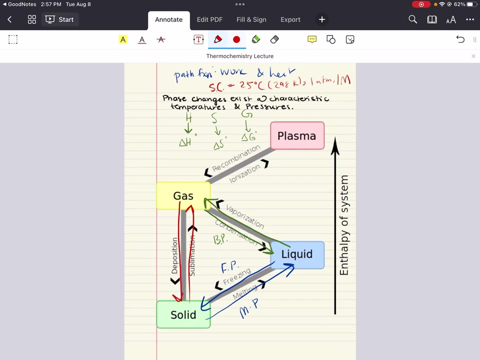 skipping the liquid state. This process is called sublimation. all right, An example is dry ice which sublimates at room temperature. all right, So that's solid to liquid. solid to gas. What gas? back to liquid Gas, back to solid. I'm sorry, That's called deposition. okay, So a gas can. 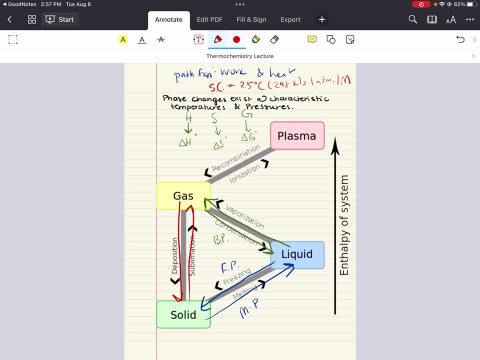 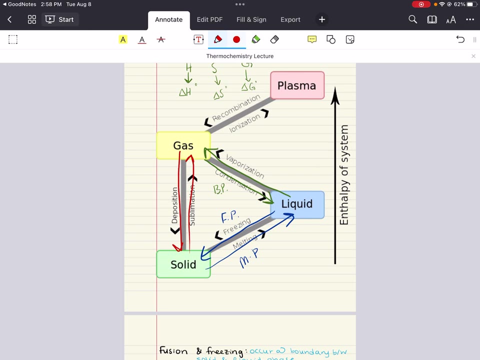 directly become a solid, Also again skipping the liquid state. this is called deposition. This is how frost forms on a cold window. all right, Deposition, Fantastic. Now those are the processes. all right, Those are the phase changes that we need to know. 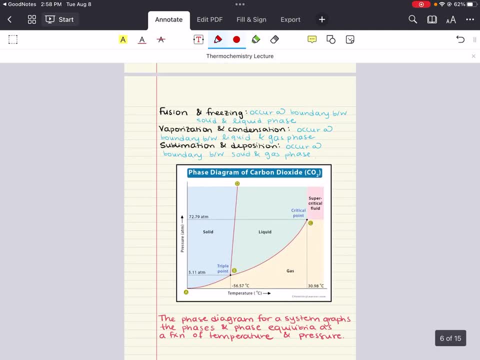 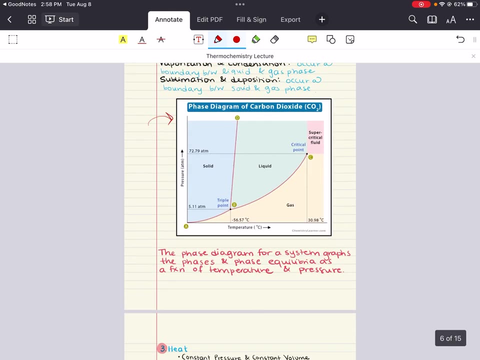 Phase diagrams, then, are charts that show the state of matter under different conditions of temperature and pressure. all right, So right, here we see a phase diagram. all right, So this is one way of encompassing this information for a specific material. So the material we're. 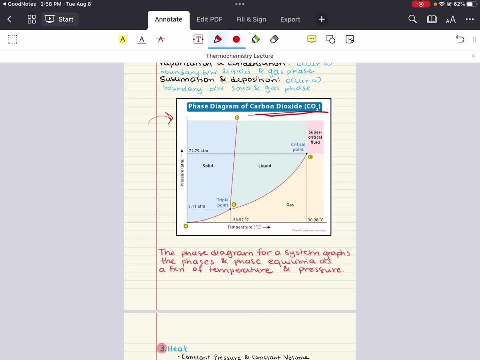 looking at here is carbon dioxide. This is a phase diagram for carbon dioxide: The x-axis represents temperature, Y-axis represents pressure, all right. And what you notice is the diagram is divided into regions that represent the different states of matter: Solid over here, all right. Liquid and gas, all right. And we see that these 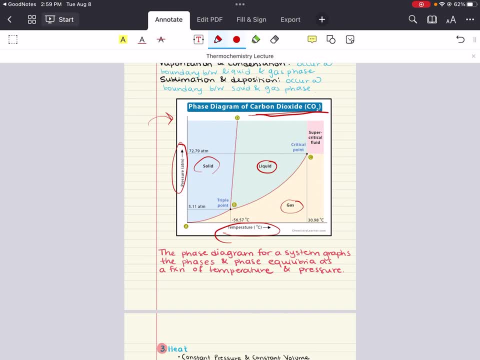 lines, separate regions, all right. There is a point right here where all three states meet, all right. This is called the triple point. It's the unique condition of temperature and pressure where all three states of matter can coexist. All right. Then there's over here. all right, This line ends right here. There's a point, This: 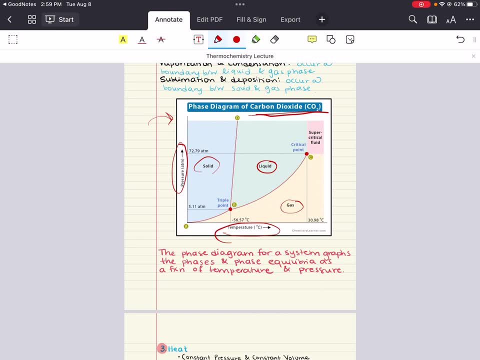 is called the critical point. It represents the highest temperature and pressure at which the substance can exist as a liquid. So beyond this point the distinction between liquid and gas phases kind of disappears and the substance now is known as a supercritical fluid. all right, 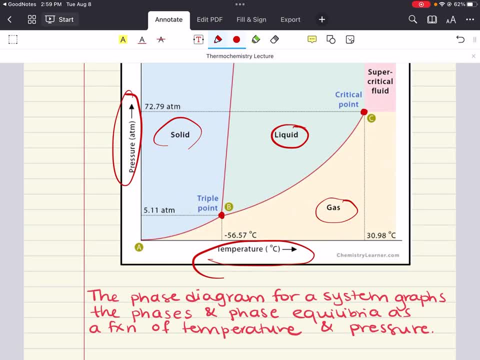 Now let's look at each of these lines. all right, There's a line here that separates solid and gas. all right, It separates solid and gas, all right. So, going from the solid state into the gas state- all right, We call this sublimation, right? We? 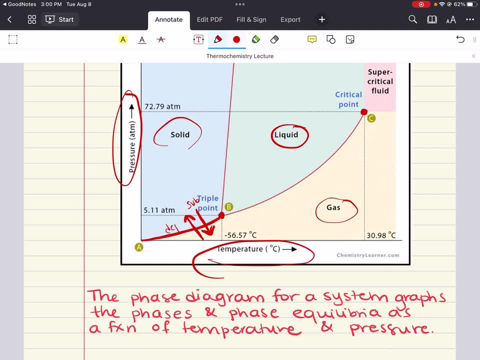 talked about this earlier- And going from gas to solid, that's deposition. So crossing any of these conditions here, you can transition under any of these conditions. passing this line that divides solid to gas, you can have sublimation or deposition, considering where you move. 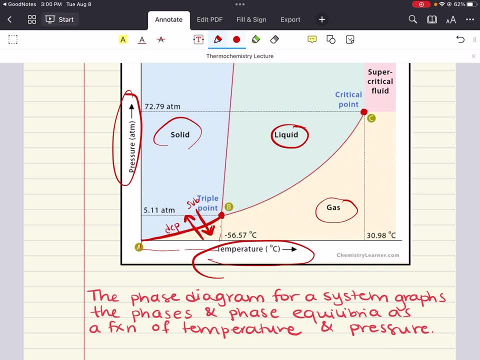 So if you move from a point right here where your temperature is minus 56.7 degrees or even lower here, minus 50 degrees, all right. And you are going to a pressure that's higher than where you are here, all right. You can have sublimation happen, all right. And if you're moving the other 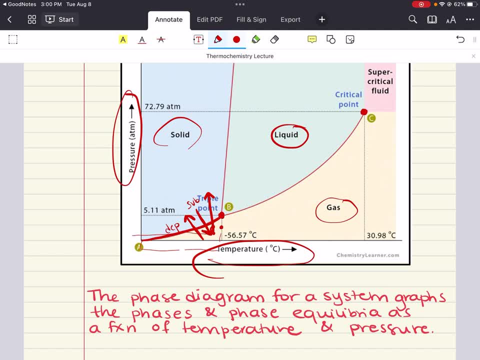 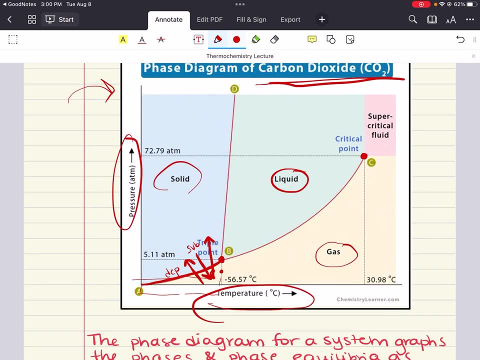 way you can have deposition. So these lines that you see divide, all right, The conditions for phases for a specific material. here this would be carbon dioxide, And passing through these conditions help you transition from one phase to another. So over here this line defines the region between solid and liquid. all right. And if 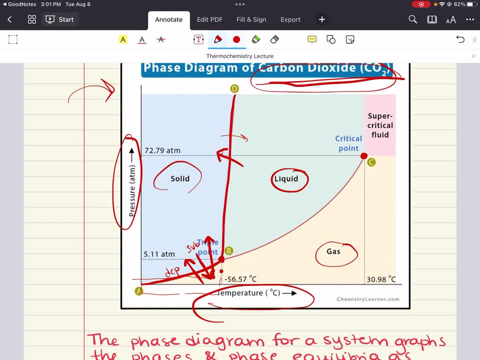 you move from liquid to solid, that is freezing. And if you go from solid to liquid, that is melting. all right, And here's the line that divides liquid and gas. All right. If you go from liquid to gas, this is vaporization. From gas to liquid, this is. 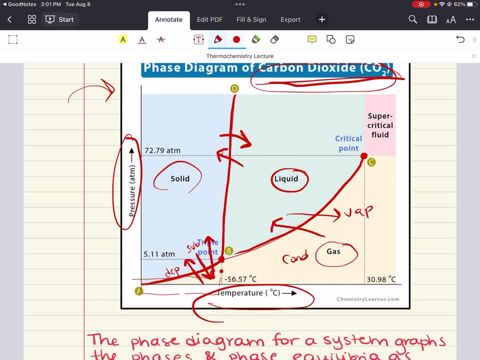 condensation, all right. So if you're at a point here, all right, and you move to conditions that are here, you're going from a gas to a liquid. all right. If you are at a condition here for carbon dioxide, so you're a liquid and you change the conditions of temperature and pressures that 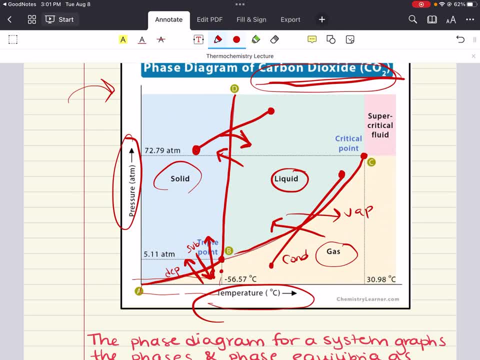 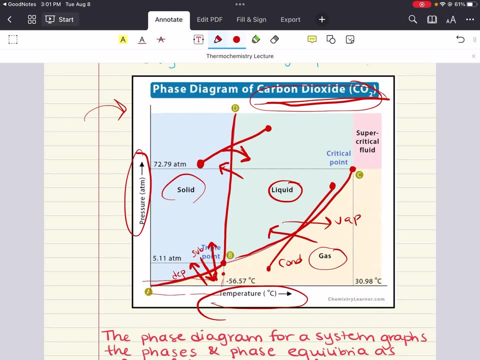 you're now here, then you are transitioning from liquid to solid. all right, So that's how you can understand this phase diagram. All right, Fantastic. And of course, remember that your triple point is where all three matters, these different states of matter, coexist, Your critical point. past it, your substance becomes. 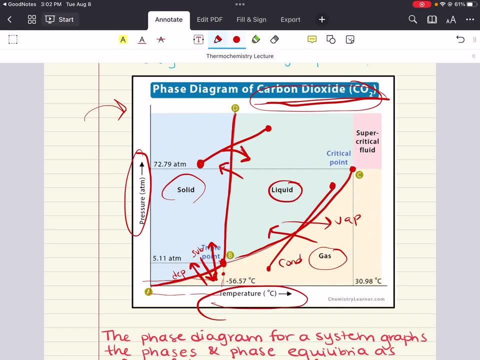 a supercritical fluid, all right, And know that the lines that divide regions like solid and liquid, liquid and gas, gas and solid- all right, you can transition between those states. all right, And we know what that's called because we covered it here. all right, Gas to liquid, liquid to gas. 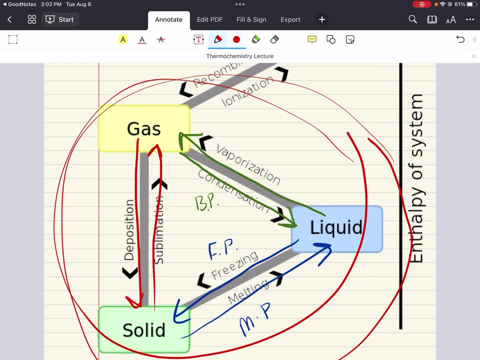 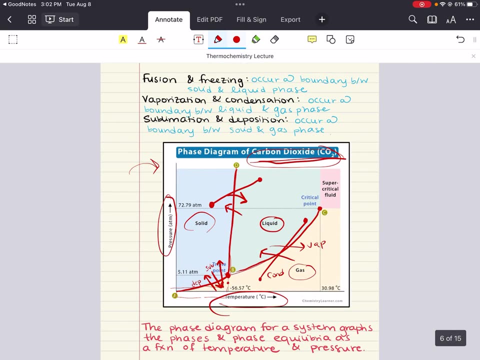 condensation and vaporization. liquid to solid. solid to liquid is freezing and melting respectively, and then solid to gas. gas to solid is sublimation and deposition- Fantastic. With that information, all right, we are prepared to move into our third objective. 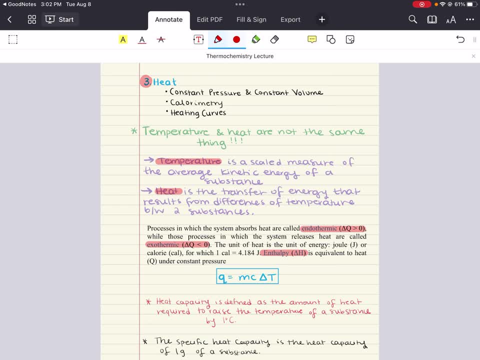 Our third objective is heat. So the first thing we want to ask here is: well, what is the difference between temperature and heat? Heat and temperature are related, but they are not the same thing. Heat is the energy that's transferred from one object to another due to a difference in temperature: Temperature. 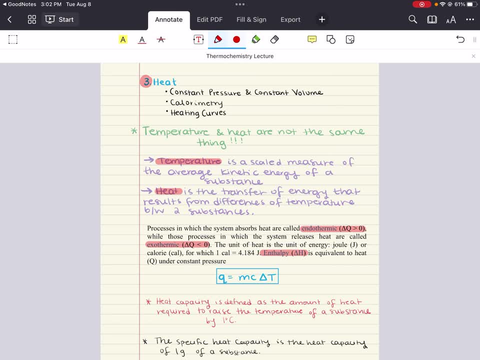 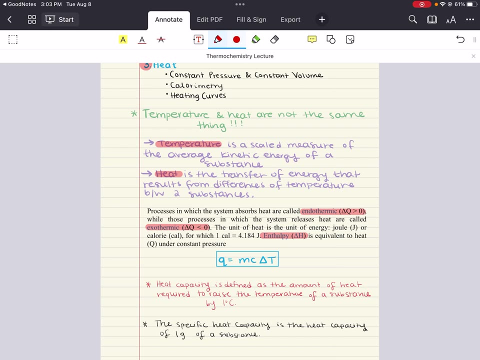 on the other hand, is a measure of the average kinetic energy of the particles in a substance. It tells us how cold or hot something is. Now, the Kelvin scale is a temperature scale starting at absolute zero, the point at which all thermal motion ceases. This is the lowest. 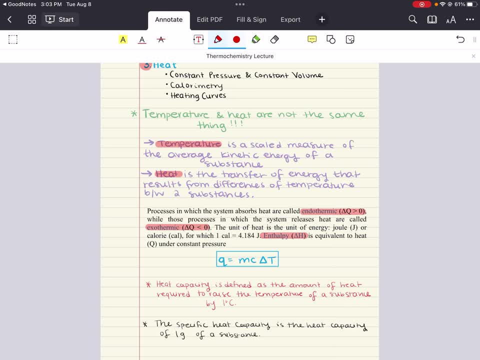 temperature possible. On this scale, the freezing and boiling point of water are going to be 273 Kelvin and 373 Kelvin respectively. all right, Now, if you have two objects, if you have two objects at different temperatures and you bring them into contact, heat will flow. 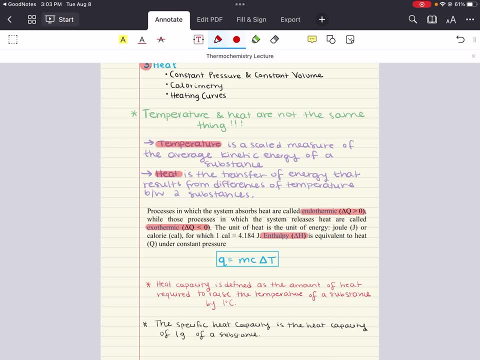 from the hotter object to the colder object. They'll eventually reach a state called thermal equilibrium, where they both have the same temperature. So if you have two objects at different temperatures, you have to bring them both to the same temperature and no more heat is transferred. 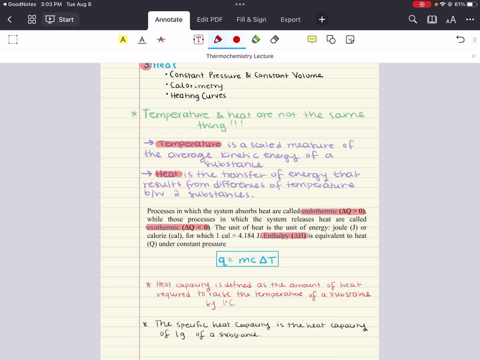 all right, Here we can start to talk about the zero with law of thermodynamics. The zero with law of thermodynamics states that if two separate systems are each in thermal equilibrium with a third system, when they are in thermal equilibrium with each other, the third system 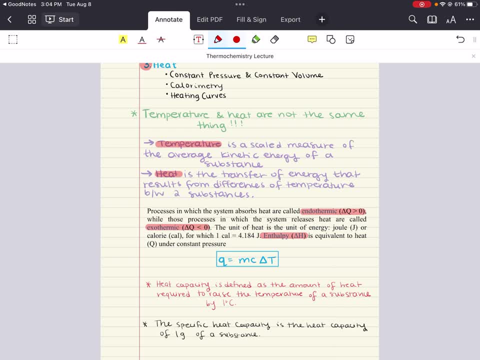 will also have all right, will also be in thermal equilibrium with the other two. So what we're saying is, if we have A—block A and block B that are in thermal equilibrium—and And block B and block C that are in thermal equilibrium, 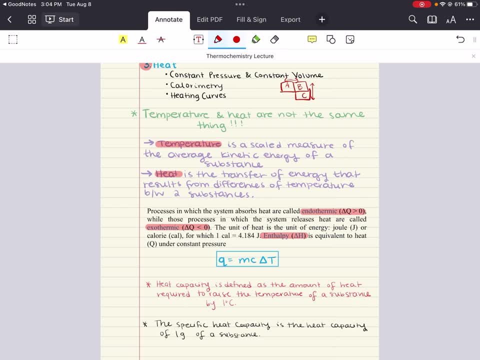 So these are in thermal equilibrium. These are in thermal equilibrium As consequenced by the zeroth law. A and C will also be in thermal equilibrium. All right, Now. processes that absorb heat from the surroundings. those are called endothermic reactions. 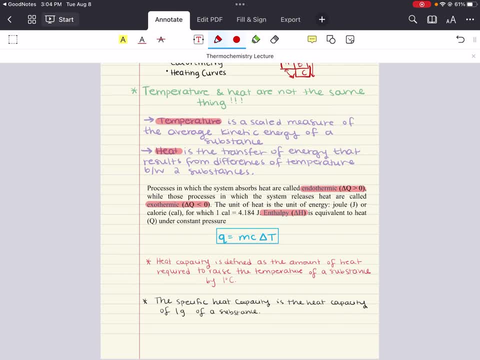 So a good example is ice melting into water. Ice absorbs heat so that it can melt into water. Therefore, it is an endothermic reaction, because it needs to absorb heat to do this. On the other hand, a process that releases heat, all right- one that releases heat, that's. 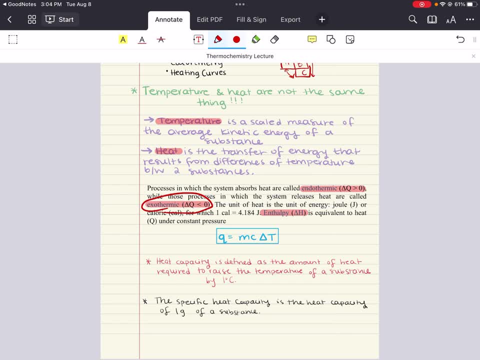 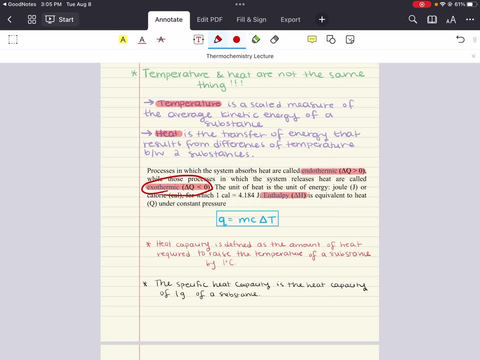 called exothermic reaction. All right Now calorimetry is a way to measure heat transfer during chemical reactions or physical changes, And there's two types. There's constant pressure calorimetry. All right, In constant pressure calorimetry, this is often done. 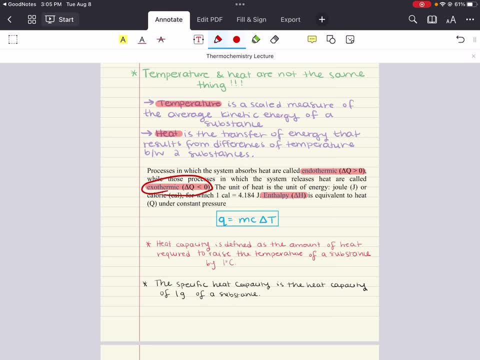 In a coffee cup calorimeter, which is essentially like a styrofoam cup. the pressure remains constant during the process, And then we can just measure the temperature change to calculate the heat transfer. All right, This method is often used in a lab setting to measure heat of reactions. 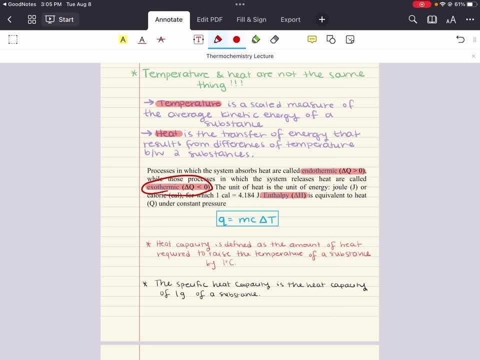 All right. Another type of calorimetry is constant volume calorimetry. This is performed in a bomb calorimeter, where the volume stays the same. We measure the temperature change, for example, in the water surrounding the vessel, And it's often used to measure heat of combustion. 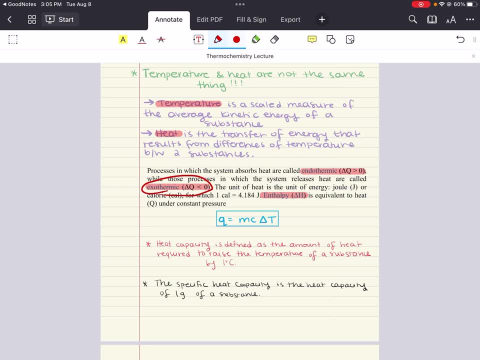 All right. The formula to calculate heat transfer is the MCAT equation. All right. Q is heat transferred. It's equal to M mass of the substance. C is the specific heat, which is how much heat the substance can absorb per unit mass. 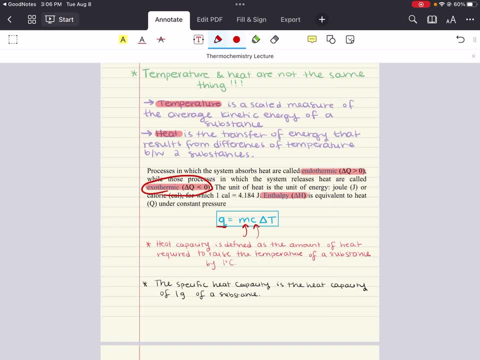 to change its temperature by one degree Celsius, multiplied by delta T, which is the change in temperature. You see how this kind of looks like It. It has MCAT, All right, This is called the MCAT equation, So heat is equal to MCAT. 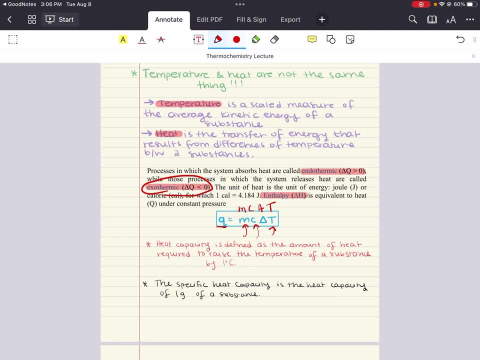 All right. Mass times C, which is specific heat times. delta T: If you know the mass of your substance, its specific heat and the change in temperature, you can calculate how much heat is transformed or is transferred. All right, So this formula is very important in calorimetry. 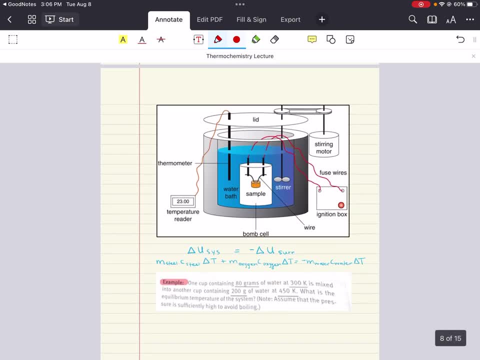 All right And specifically, we can actually start to think a little bit more about bomb calorimetry. The bomb calorimeter, which is the setup that you see here, is a device that's used to measure the heat of combustion of a sample. 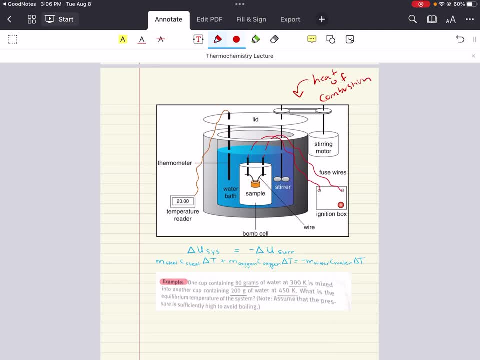 All right. It consists of a strong sealed container right here, which is the bomb part, which is placed inside a larger container that is filled with water, like you see here. All right, The sample, usually something like a hydrocarbon, is placed inside the bomb and then filled with water. 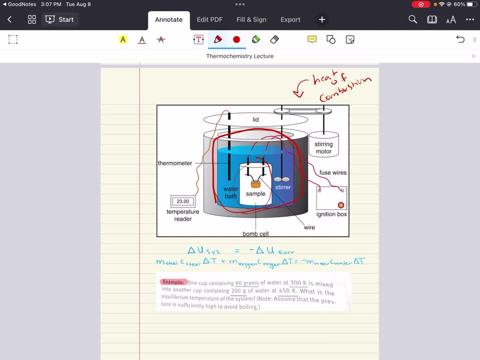 All right. And then filled with pure oxygen and ignited- All right. And the heat produced by the combustion reaction is absorbed by the water- All right, It's absorbed by this water and that's going to cause a change in the temperature. 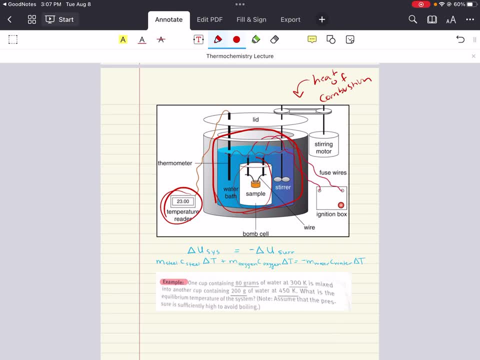 All right. It's going to cause the temperature to rise and you can measure that. A bomb calorimeter is insulated in a way that no heat is exchanged with the environment. That's why it's called an adiabatic process. All right. 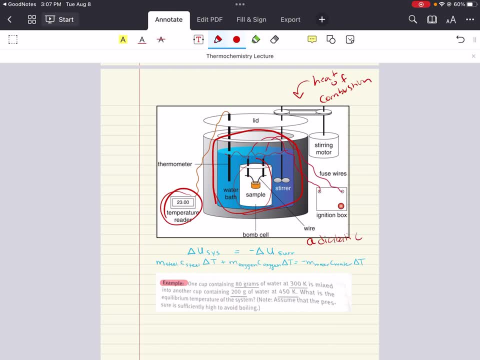 A bomb calorimeter is an adiabatic process. All right, So all the heat generated from the burning sample, it stays within the calorimeter system. All right, Then the total change in internal energy of the calorimeter, which includes the burning. 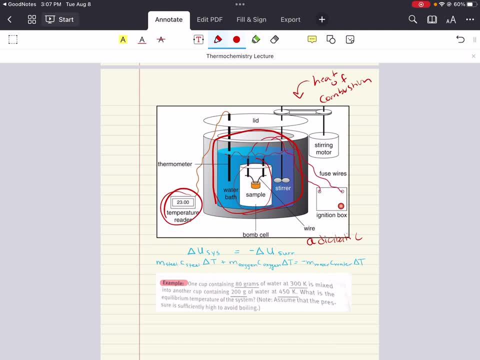 sample and the water is going to be zero, And this is because the energy released by the burning sample, which reduces its own energy, is absorbed by the water in the calorimeter and that's going to increase its energy. So this is a clear depiction of conservation of energy. 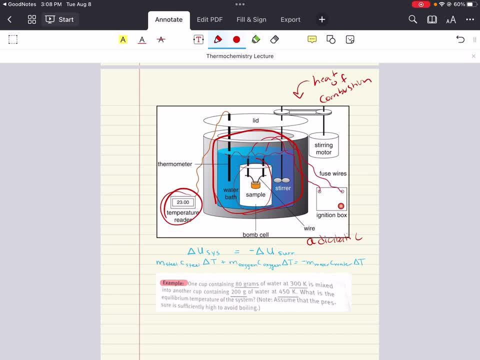 Now, since no work is done because the volume is constant, all right, and the burning sample doesn't move or exert force on its surroundings and there's no heat exchange with the environment, any change in the energy of the water is exactly equal to the negative change in the energy. 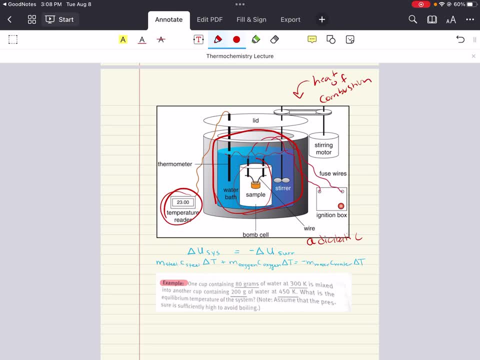 of the sample. All right, And so, in simple terms, the heat gained by the water is the heat lost by the burning sample. All right, And so, by measuring this temperature rise Of the known volume of water, we can calculate the heat released by the combustion reaction. 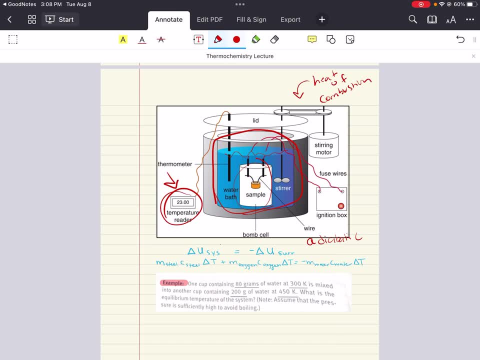 and we can therefore write the following relationships: The delta U of the system is equal to the minus delta U of the surroundings. All right Now, because no work is done, the heat of the system is equal to the minus heat of the surroundings. 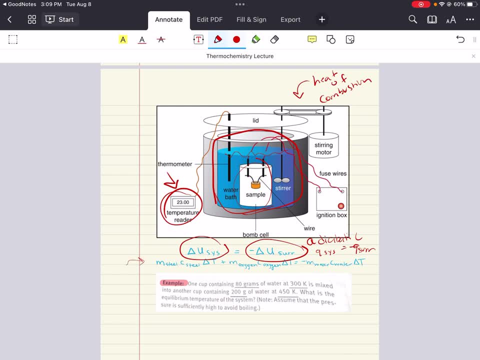 All right, And then that means we can write an MCAT equation relationship for the whole bomb calorimeter. All right, We can write: MCAT for the steel plus the MCAT of the oxygen that's ignited is going to equal the MCAT equation for water. 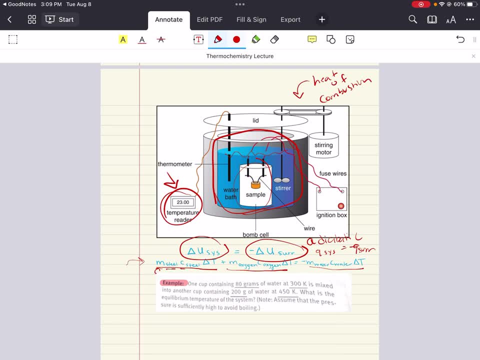 So M for the mass of the steel times, the specific heat for the steel times, the delta T plus the mass of the oxygen specific heat capacity, specific heat for oxygen plus delta T, is all going to equal the minus mass of the water. specific heat of the water times, delta T. 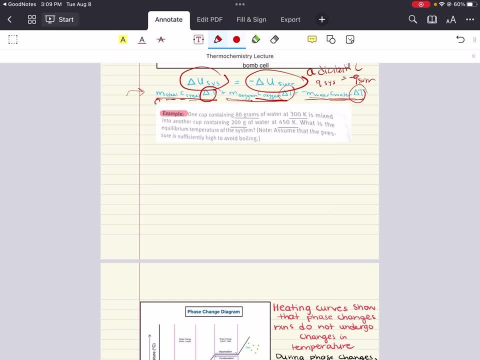 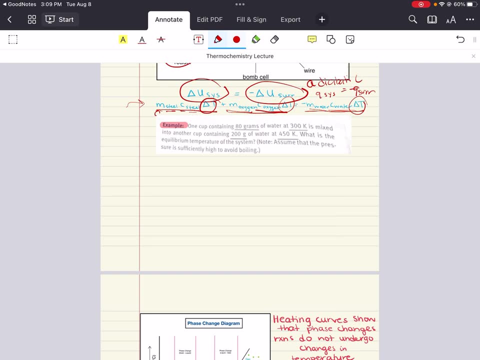 All right, And we can go ahead and do an example problem to make sure That we understand this. This problem says: one cup containing 80 grams of water at 300 Kelvin is mixed into another cup containing 200 grams of water at 450 Kelvin. 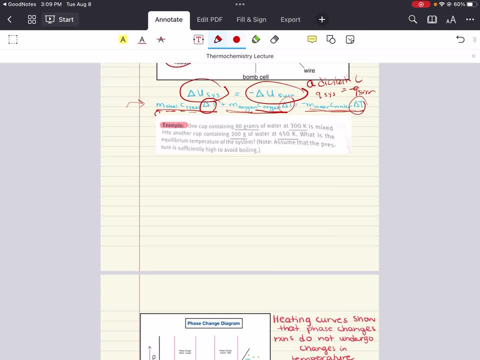 What is the equilibrium temperature of the system? All right, Assume that the pressure is sufficiently high to avoid boiling. All right. So the two liquids undergo thermal exchange, And so the heat given off by one liquid has to be equal to the heat absorbed by the other. 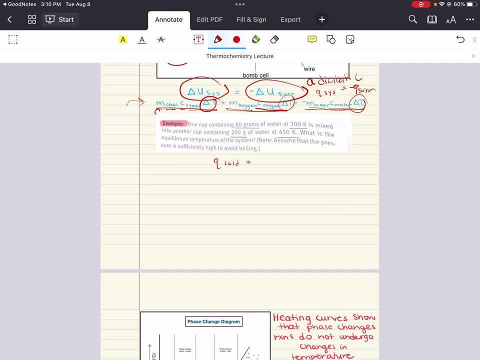 And so we can write that the heat for one, say the cold one, is equal to the minus heat Heat of the hot one. All right, And then we can change this All right Into an MCAT expression: right, The mass for the cold times, for the cold water times, the specific heat for water times, delta. 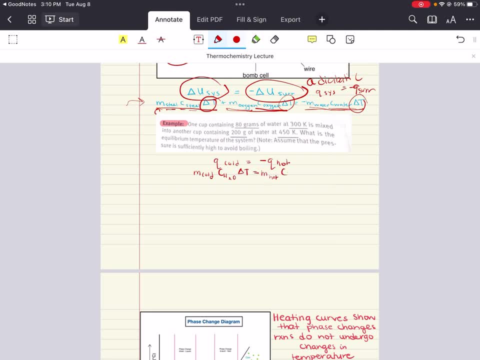 T is going to equal the mass of the hot water. specific heat of water dealt, minus, minus delta T hot. All right, This is minus delta T- cold. All right. Now we can plug in the values from the question And because we are solving for final equilibrium temperature of a mixture, we can use any value. 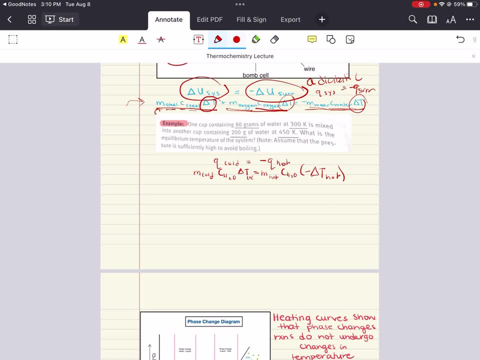 of C, as long as we are consistent for both liquids. So in this case we have two quantities of water, So we're just going to use the specific heat for water, which is just one calorie over gram per Kelvin. All right, So one for H2O is one cal per gram per Kelvin. 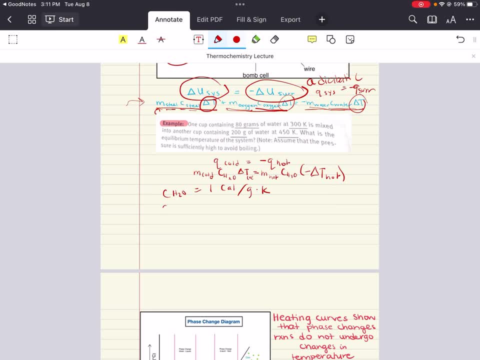 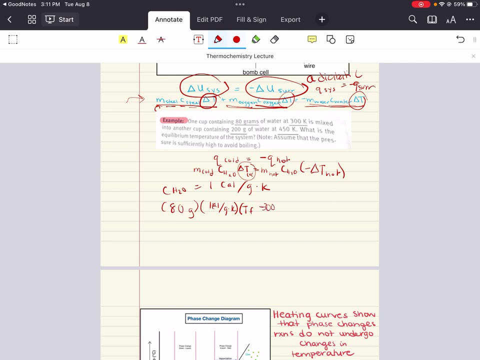 All right, So we're going to go ahead and plug in values here. M cold: 80 grams Multiplied by one cal per gram per Kelvin: All right, Here it's final temper for delta. T cold is going to be T final minus 300 Kelvin. 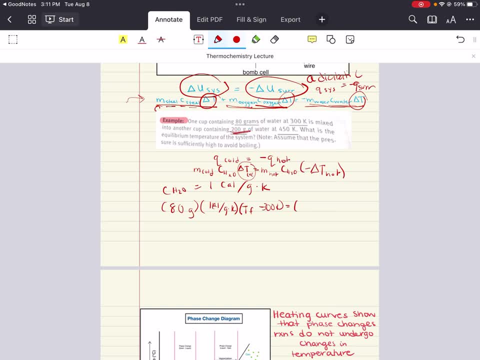 That's going to be equal to the mass of the hot water, which is 200 grams, All right Again, multiplied by the specific heat: one cal per gram per Kelvin, All right, And here we're going to have T. final is 450 minus T cold. 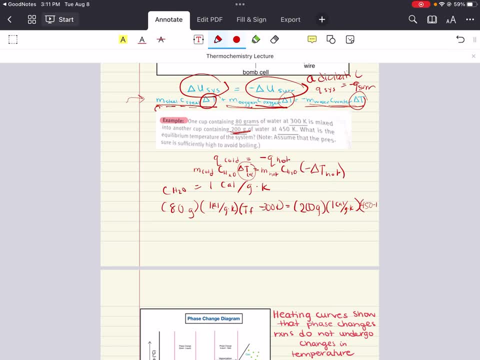 Minus T final. All right, I mean, this is the initial temperature, minus T final, and this is switched up like this because there's a minus sign here. All right, So what we can write now is that 80 Tf. all right, that's multiplying the 80 by the Tf. 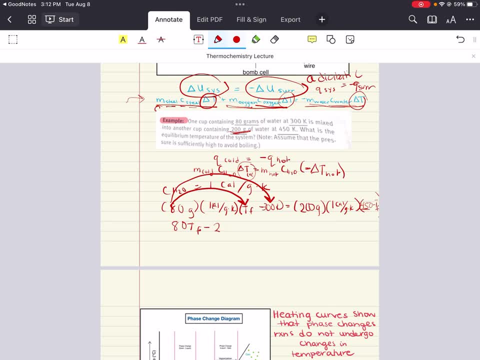 And then we multiply the 80 by 300.. So minus 24,000 cal is equal to now the 200 multiplied by 450 and also multiplied by Tf. So 200 times 450, that's about 90,000 cal minus 200 Tf. 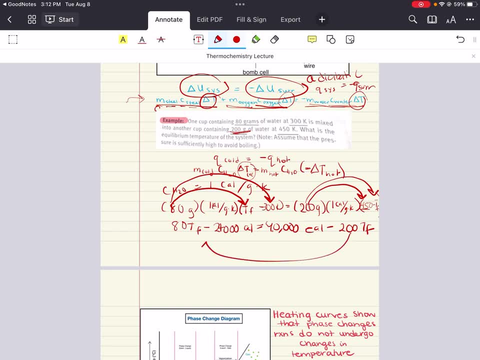 All right, Now we want to move all the Tf's to one side and all the calories to the other side. All right, So we're just going to do that. We're going to move the, we're going to add 200 Tf to both sides. 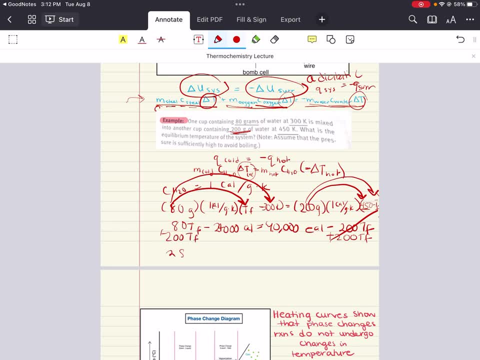 So that cancels out and we add it here. So now on one side we have 280 Tf, All right, And that's equal to: We're going to add 24,000 to both sides. This cancel out and this is 24,000. 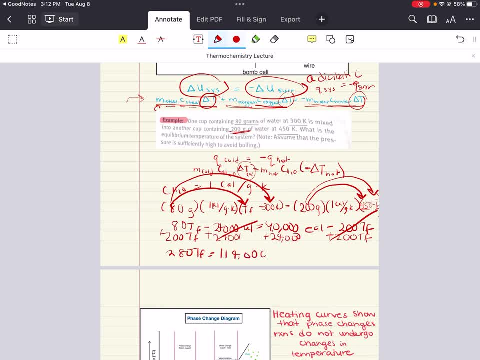 And so that is 114,000.. All right, And to solve for Tf is just going to be 114,000 over 280, which is approximately 400 Kelvin. It's actually like 405, 407,, all right, but approximately 400 Kelvin. 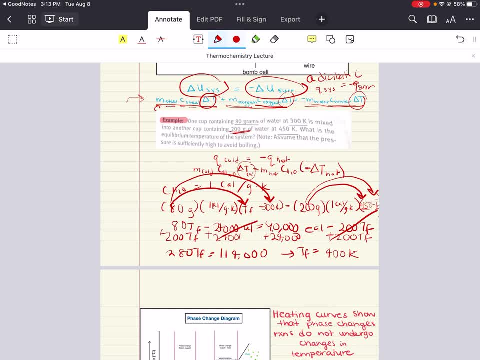 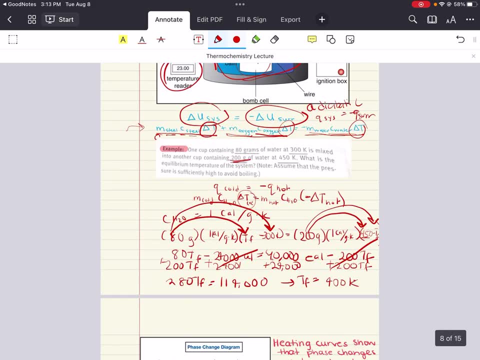 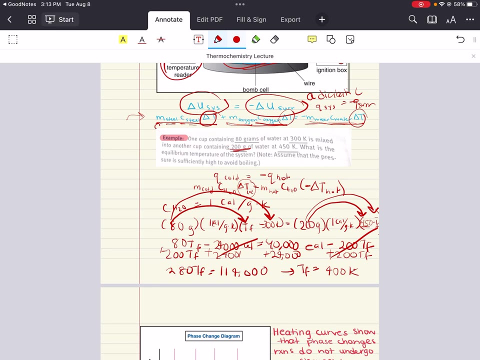 All right, And we figured out what the final temperature was Using. Okay, So what we learned in regards to how to calculate heat and how to calculate heat for two systems? All right, Like in this problem, what is the equilibrium temperature of the system? 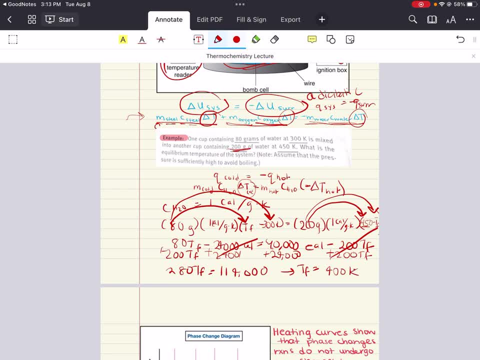 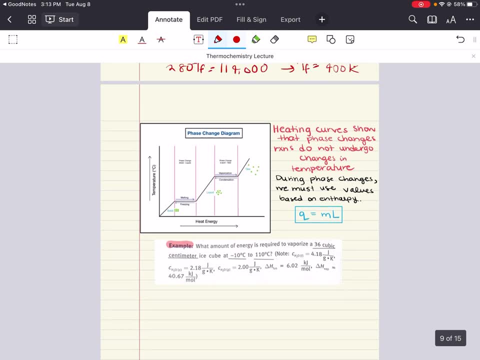 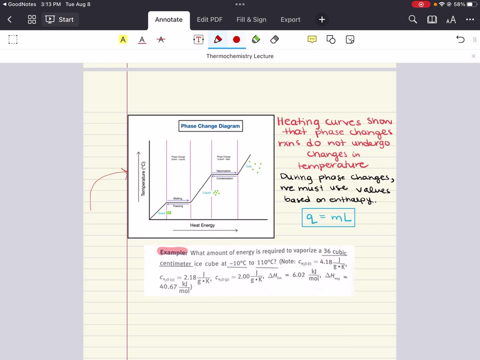 That final temperature. we were able to solve that. All right, Fantastic, Awesome. Now we can also look at heating curves here. All right, This is a heating curve, a phase change diagram, All right. So this is where the X axis is the heat added. 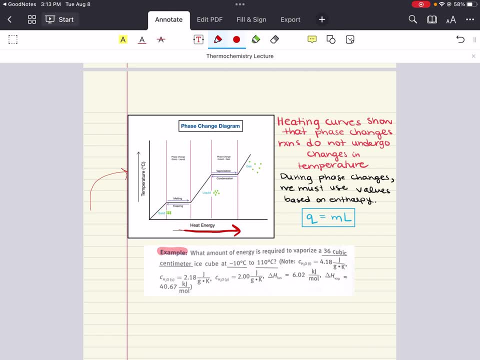 Y axis is temperature. Now, when a compound- all right, if we're starting here as a solid- when a compound is heated, the temperature rises, rises, rises until it meets or reaches the melting or boiling point, All right. Then the temperature kind of remains constant as the compound is converted to the next phase. 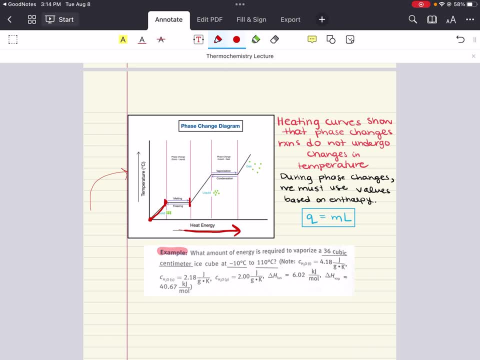 All right. Once the entire sample is converted, then the temperature starts to rise again until it reaches, All right, The next phase, transition, All right, And then it stays constant, All right, Until the all the sample is converted to the next phase. 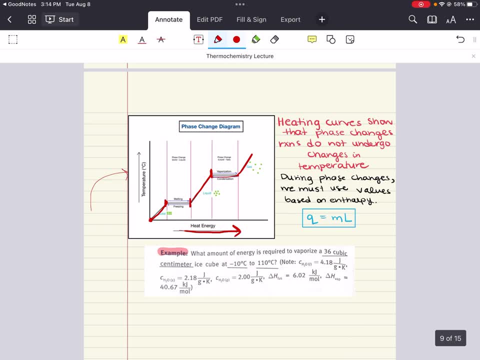 All right. And then it increases the temperature. All right. So heat curves, they show that phase change reactions, they do not undergo changes in temperature. All right For certain parts. All right Here, when you reach. when you reach the point where 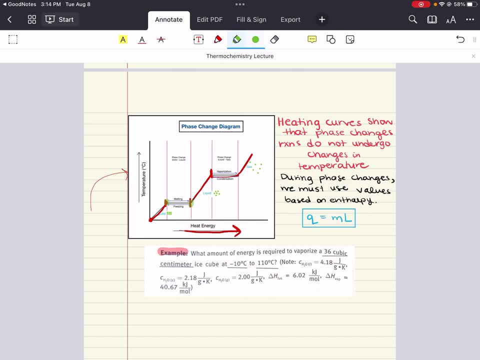 Um, yeah, your solid is melting into your liquid. All right, This melting point, All right. There is no change in temperature as all the solid begins to slowly convert into liquid. All right, The temperature will only start changing again after all the solid has converted to liquid. All right, So at this. 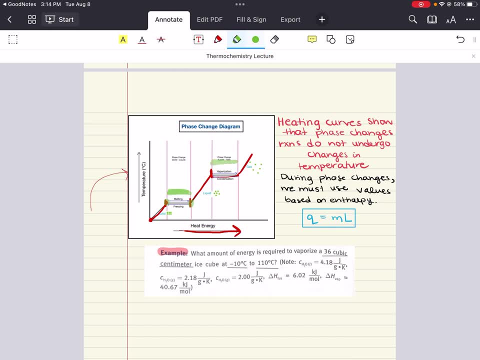 point. all right, there is no change in temperature. It's the same here when the phase change happens between liquid and gas. What does that mean for us? What this means for us is right here. we cannot use the MCAT equation to calculate heat transfer. We have to use a different. 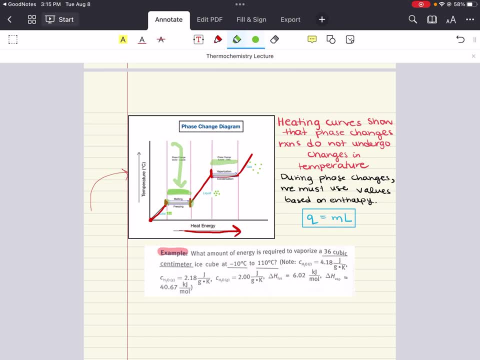 expression, And this expression is that heat transferred is equal to M times L, where M is the mass and L is the latent heat, which is a general term for the enthalpy of an isothermal process, And it's given in units of calories per gram. So, in essence, during phase changes, 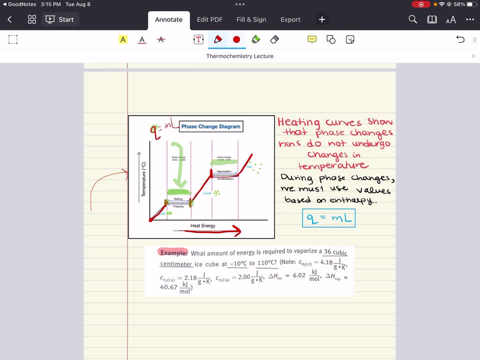 we must use values based on enthalpy. So when you're transitioning at the solid liquid phase right here, the enthalpy or the heat of fusion, delta H fusion- all right for changing between solid and liquid, that's what we call it- It must be used to determine the heat transfer during the 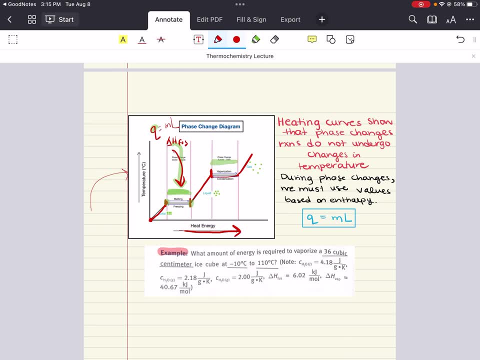 phase change And then, when transitioning from solid to liquid, the change in enthalpy is going to be positive because heat is being added when transitioning from solid to liquid, When you're transitioning from a solid to a liquid. but then, if you're transitioning from a 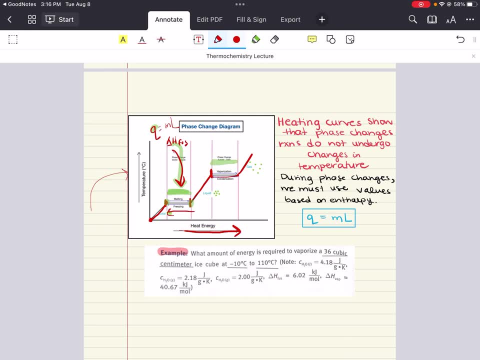 liquid to a solid, all right. the change in enthalpy is going to be negative because heat has to be removed Now at the liquid gas boundary, the enthalpy or heat of vaporization. delta H vape- all right- has to be used here. All right, And it's sign convention follows a similar pattern. 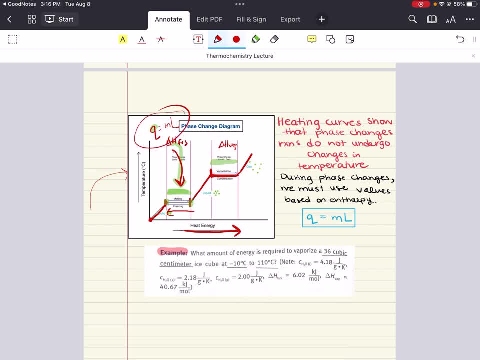 And again we use this expression- Heat is equal to M mass times, L latent heat, which is a general term for enthalpy. So it can be delta H fusion If you're talking about solid to liquid or liquid to solid, and it will be delta H vaporization If you're going from liquid to gas or gas to liquid. 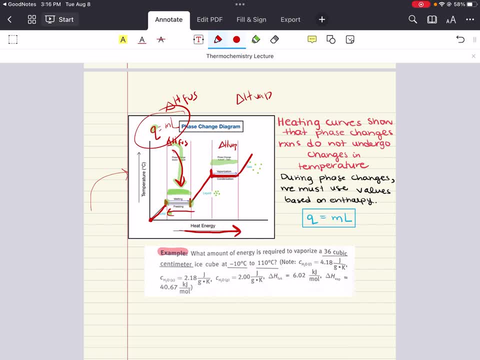 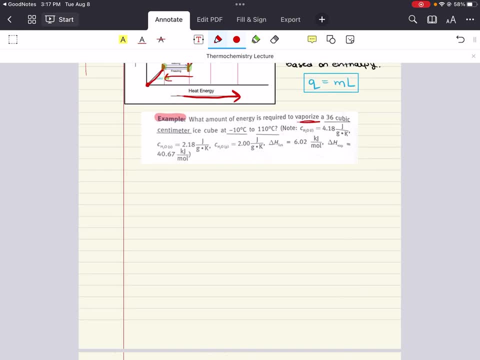 All right, let's do a quick problem. This problem says what amount of energy is required to vaporize a 36 cubic centimeter ice cube at minus 10 degrees Celsius to 100 degrees Celsius. All right, And we're given a lot of information. 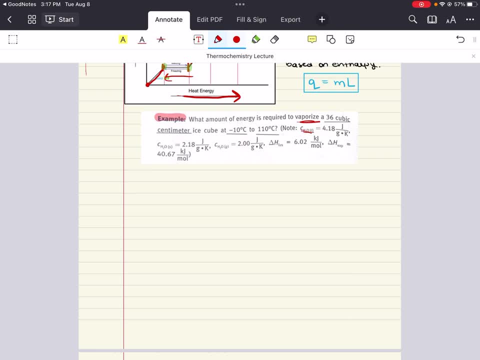 here. Specific heat of water- All right. Liquid specific heat of water. solid specific heat of water gas. delta H fusion and delta H vaporization: All right. We need to know what amount of energy is required to vaporize 36 cubic centimeters of ice cube. So we're going from solid water. 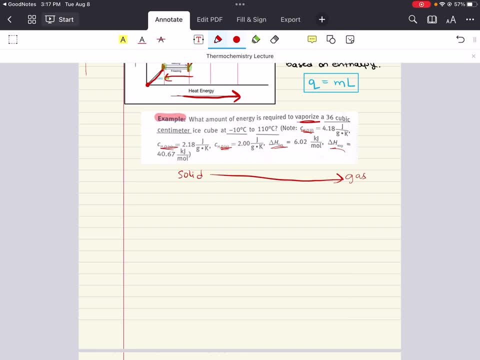 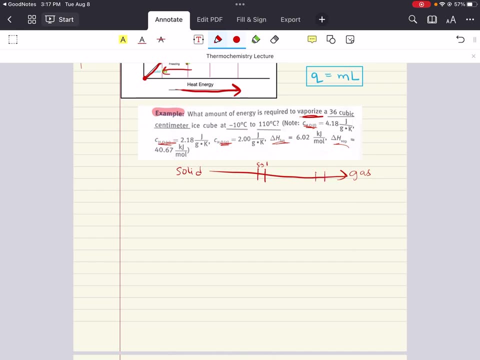 all the way to gas, All right. And so it's going to pass a solid to liquid boundary and then it will pass a liquid to gas boundary to be able to do that, All right. So we can visualize it like that. We can visualize that. 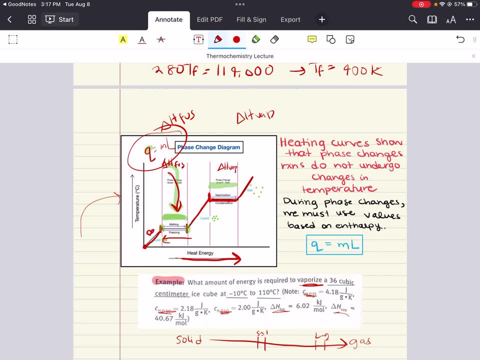 the process it's going through is from solid to liquid, is from solid to gas, So it's going to go through a phase change diagram that looks like this: All right, Now recall that one cubic centimeter is equal to right. This is given to us in cubic centimeters. 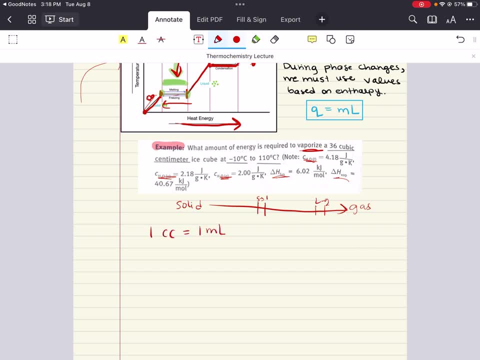 One cubic centimeter is equal to one milliliters, And that water at STP has a density of approximately one gram per milliliter. All right, Now some of the constants given are in terms of mass grams and some are in terms of mole, So we should definitely convert the mass to moles. 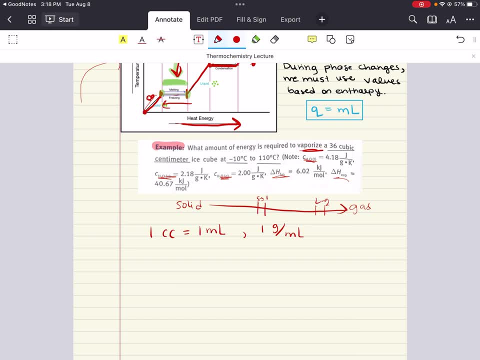 All right, We have 36 grams, All right, And we want to convert that to moles. So N is equal to 36 grams H2O. All right, And we're going to convert it to moles. So we are going to use dimensional analysis. Water is about 18 grams per one mole And this is going. 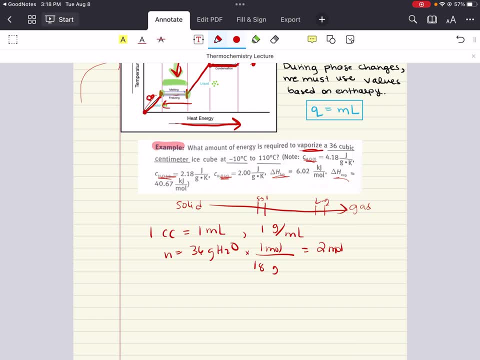 to give us two moles. Now, because we are beginning in the ice phase, we must heat the ice cube to the solid liquid phase transition first, which occurs at zero degrees. So our first step involves a change in temperature. So we must first heat, So we must first use a heat formula that contains 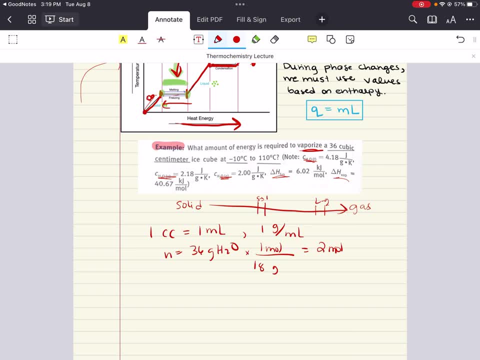 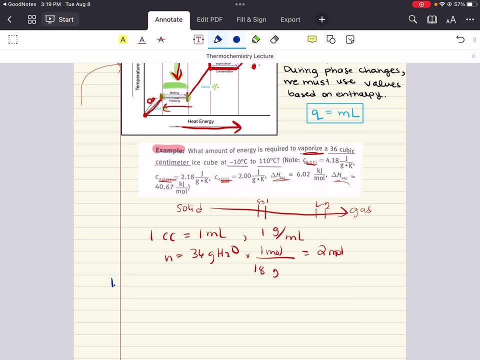 delta T and all its variables. So first things first. All right, Our first step, if we're trying to ultimately go from solid to gas, our first step is to go from solid to liquid, All right, And to reach that boundary, All right. So our first step is going. 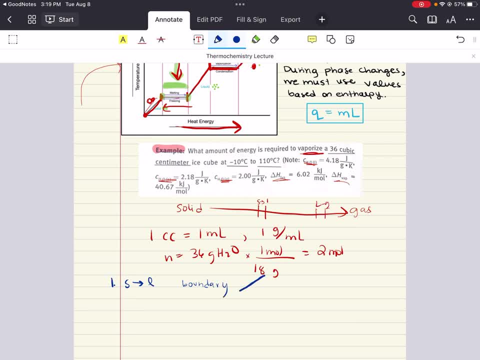 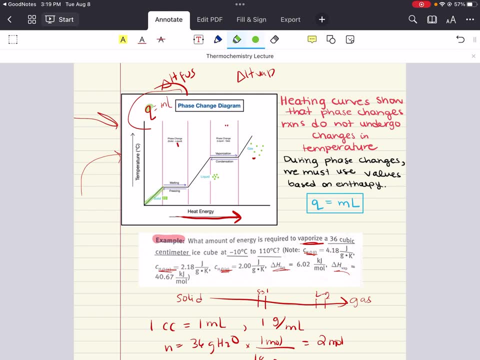 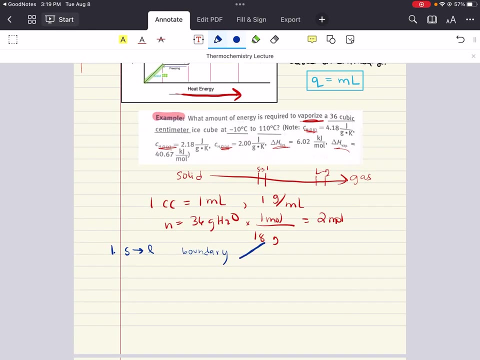 up in our graph. All right, Like right here, I'm going to highlight it as we go. All right, Our first step that we want to calculate is this process, right here, going from solid to this point, All right, Where fusion can happen. All right, So that first part. 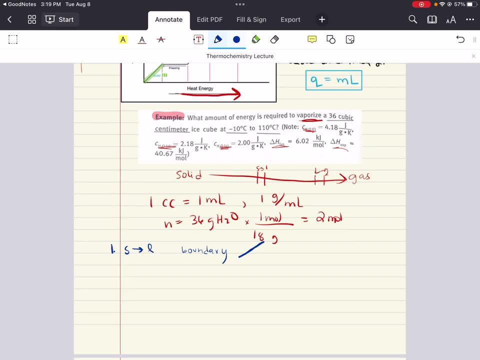 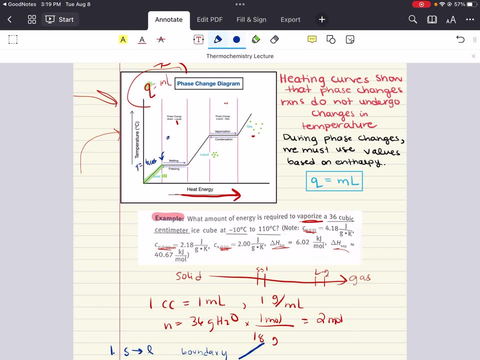 from solid to liquid. we have to calculate that, All right, And that first part we're going to use. we use our MCAT equation right here. All right, We use our Q equals MCAT here. Here, at the boundary, we use QML. Now we're calculating this first part, So we're going to use our MCAT equation. 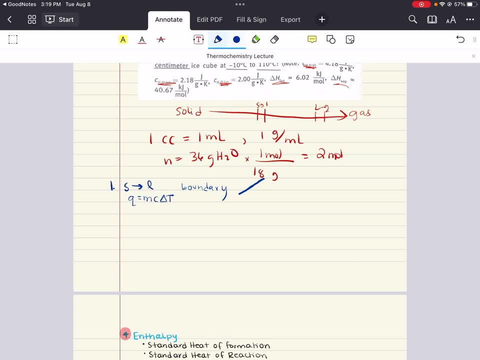 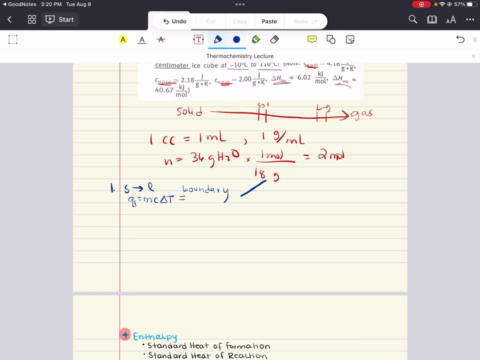 Q equals MC delta T. All right, We're going to call this Q1.. All right, So this is going to be the mass of ice, specific heat of ice, delta T. All right. Mass is 36 grams. The specific heat of solid is 2.18.. 2.18 joules grams. Kelvin, Beautiful Delta T, which they say. 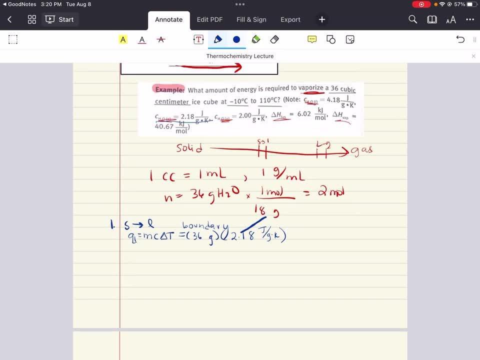 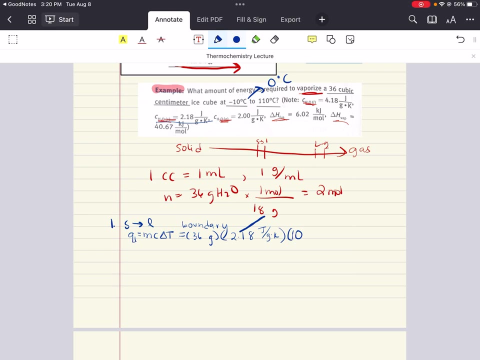 10, which is going from minus 10 degrees Celsius to zero degrees Celsius. Right, Because that's the melting point here. All right, So zero degrees, So from minus 10 to zero, And so the delta T here is 10.. All right, 10 degrees Kelvin, 10.. 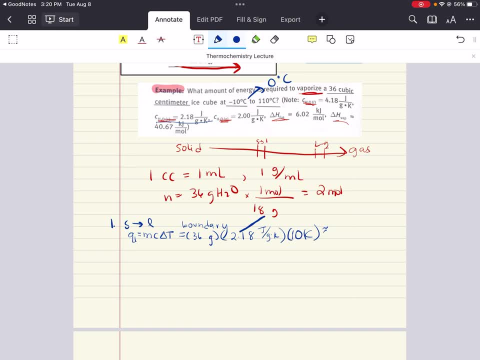 Kelvin, I should say: All right, This is going to be 36 times about two about multiplied by about 10.. So this is approximately 720 joules. All right, Or that's also equivalent to 0.72 kilojoules. 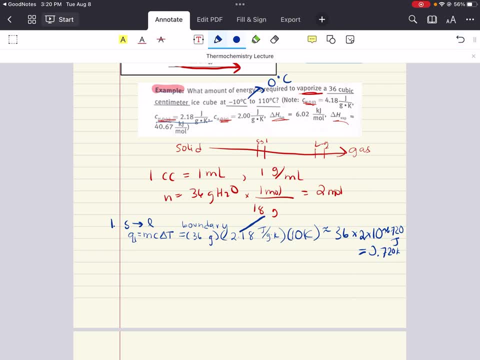 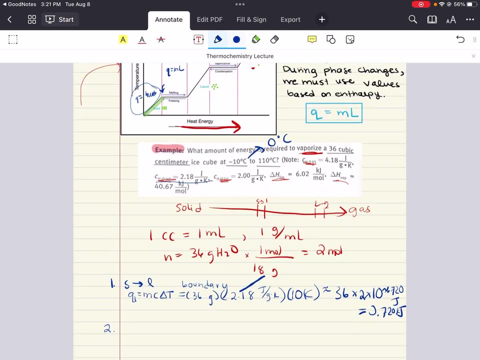 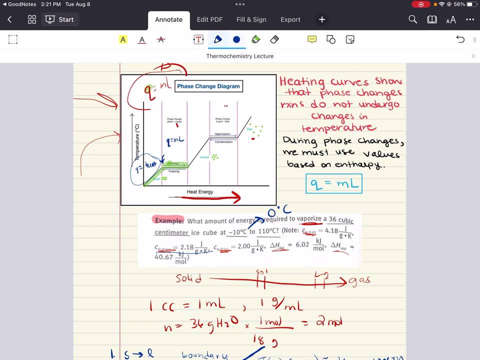 Kilo joules, All right. So that's our first step. Now, in our second step, what happens in our second step? then we're at this boundary, right here, Of melting, All right. So we need to calculate how much heat is consumed in this step. So we 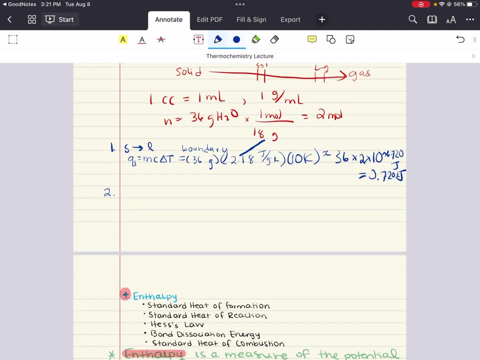 have to use Q equals ML for the second step, because we're in the boundary of solid and liquid here, Boundary, Boundary, All right. So we have to use: Q is equal to ML, All right. Here we're going to use All right, Because L is our latent heat and this is between solid. 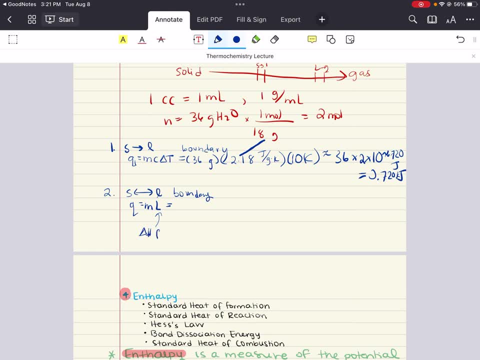 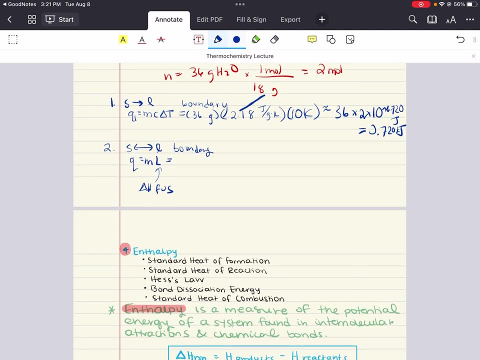 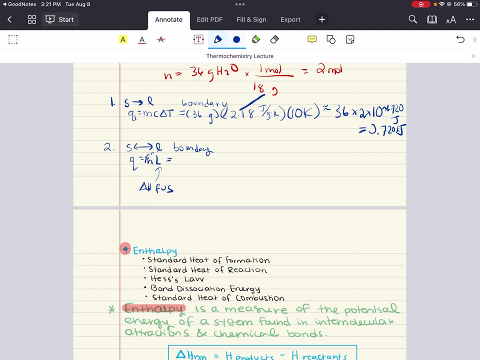 and liquid. So it's delta H of fusion, And this variable is given in kilojoules per mole. Our mass should be. we can use moles instead of mass here, so that the units cancel out appropriately, All right, That's why we. 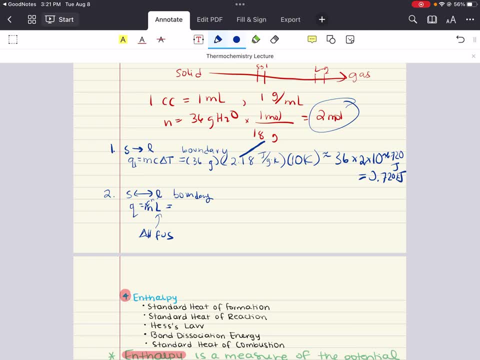 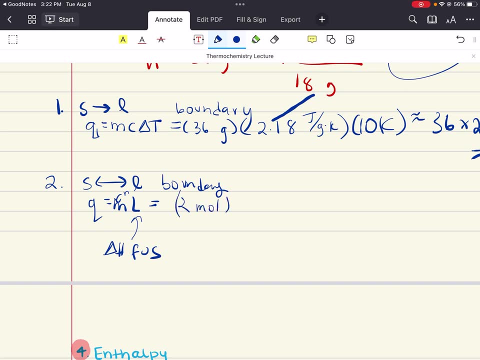 calculate two moles earlier so that we can use it for this step. the Q equals ML steps, So we can write here two moles. All right, Two moles multiplied by the delta H of fusion which is given to us above It's 6.02 kilojoules per mole. 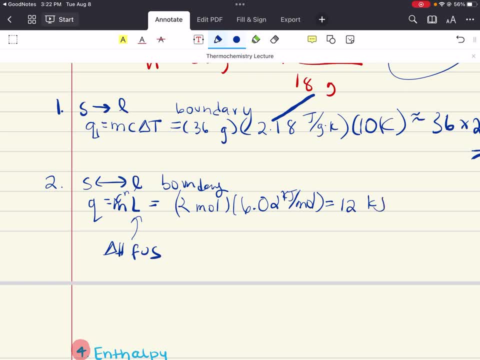 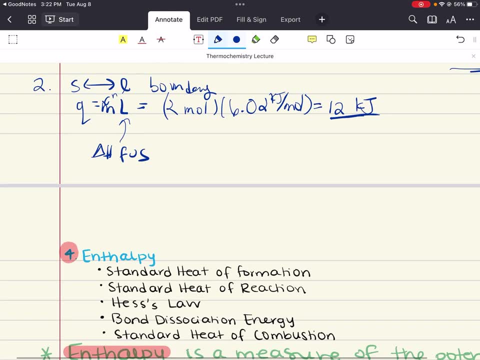 All right, And that gives us about 12 kilojoules. All right, And we want everything in kilojoules so that we can sum it up properly at the end. All right, Then we can go to step three, Step three. 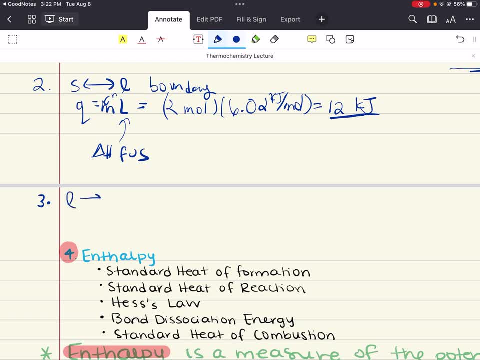 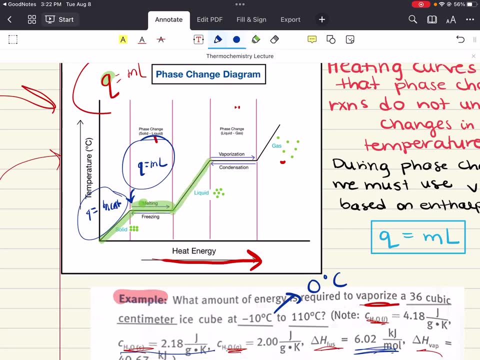 is when we go. we're now all liquid and we're heating up to get to gas. All right, So we're right here in the graph now, Liquid trying to go to gas. Here we use our MCAT equation: Q equals MC delta T. All right, So that's what we're going to use to calculate this portion of. 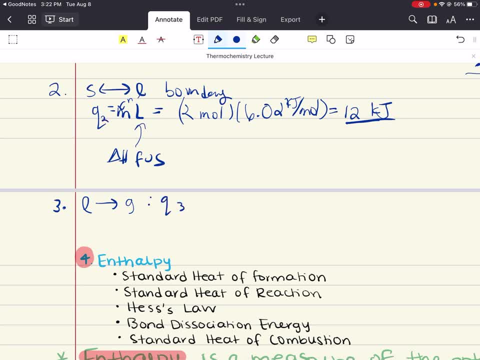 the process. So Q3, so that was Q2.. This is Q3- is equal to M water, C water of liquid, minus delta T. All right, This is going to be 36 grams multiplied by 4.18 joules per gram per Kelvin. That's what we're. 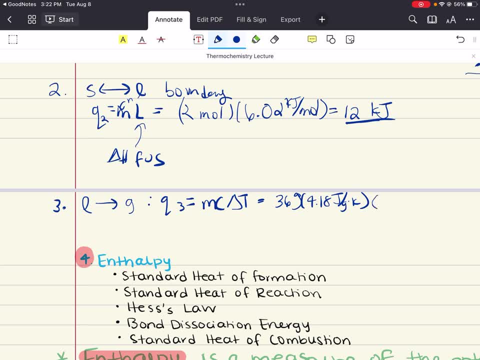 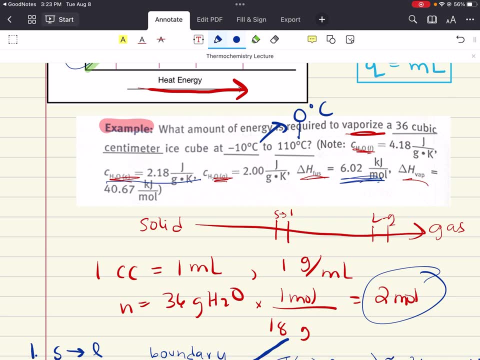 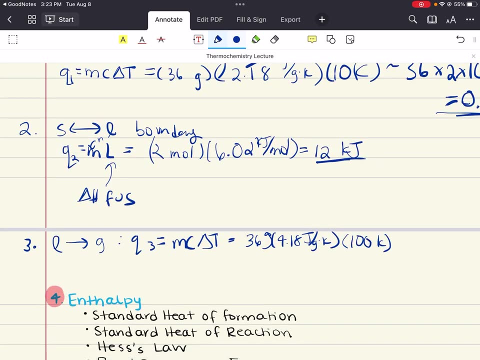 given in the problem for liquid water, All right. And then we're going from zero to a hundred. We're going from zero now to about a hundred, All right, Cause that's where the boiling point is All right, And that's a change of 100 Kelvin, All right. And if we multiply this it's about 36. 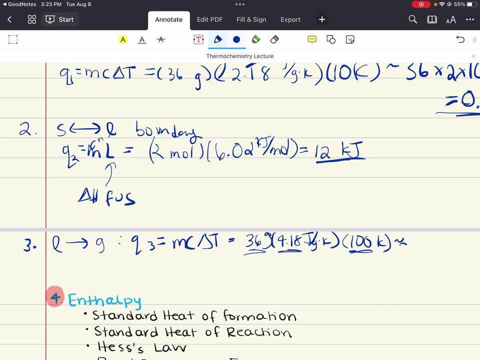 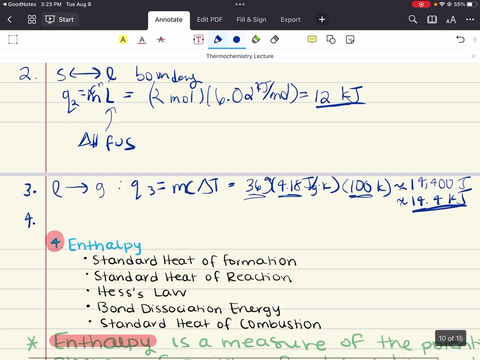 times about four and a hundred, So those are easy numbers. to multiply That gives us about 14,400 joules, And that is approximately 14.4 kilojoules. Again, we want everything in kilojoules, so we can add it up nicely. All right, Then we're at 0.4.. All right, Now we're at this boundary. 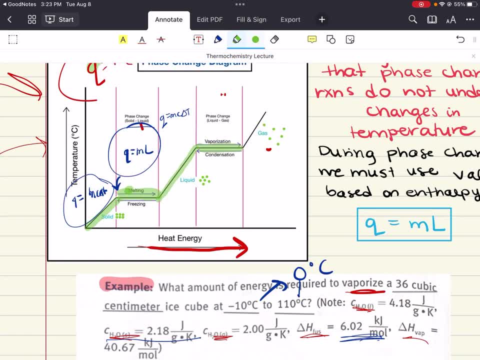 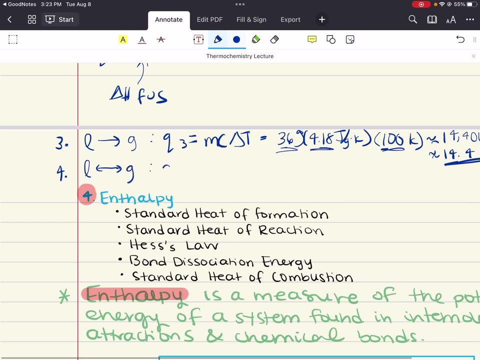 of vaporization, All right. Trying to heat up everything That is a liquid, to turn all of it into gas, Here we use our Q equals ML equation. All right, So now we're at the liquid gas boundary. All right, We use Q equals ML, except for M. 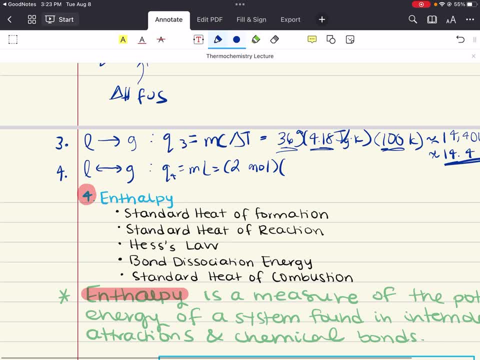 we're going to use moles, So things cancel out. So two moles times L: here is now delta H of vaporization. All right, We were given that it's 40.67 kilojoules per mole, All right, And that. 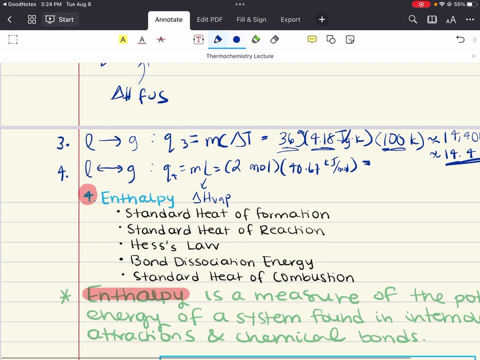 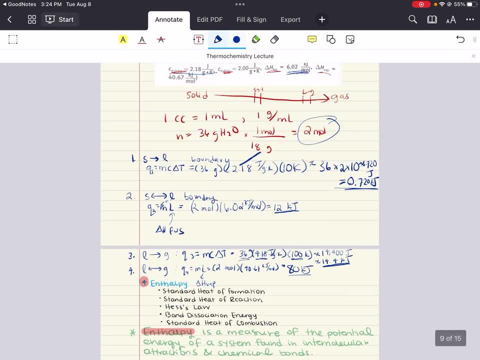 gives us approximately- think about it two times 40, that's 80 kilojoules. 80 kilojoules, Nice. Now remember, we're heating up all the way to 110.. So here, when we reach this, this is still. 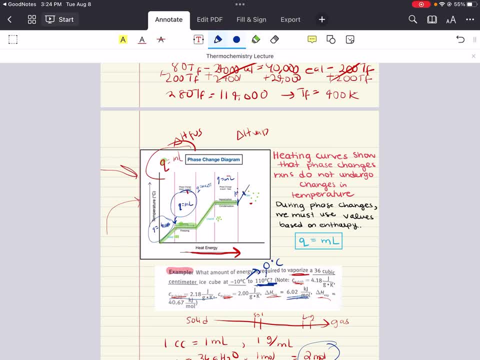 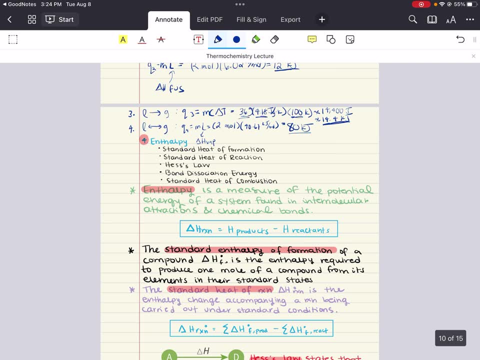 about a hundred degrees. So we're still- you know, we're also have to calculate this process right here. All right, From a hundred to 110.. So we have a fifth step- All right, Where we use our MCAT equation. All right, Except now.